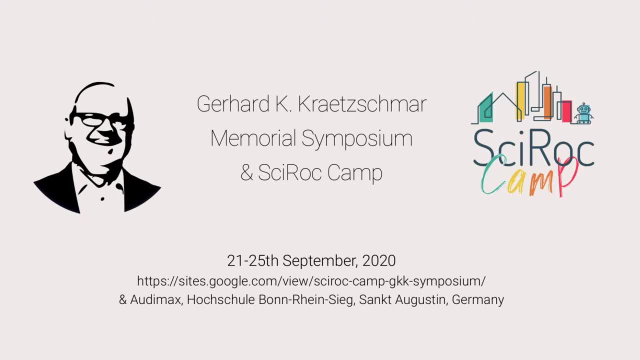 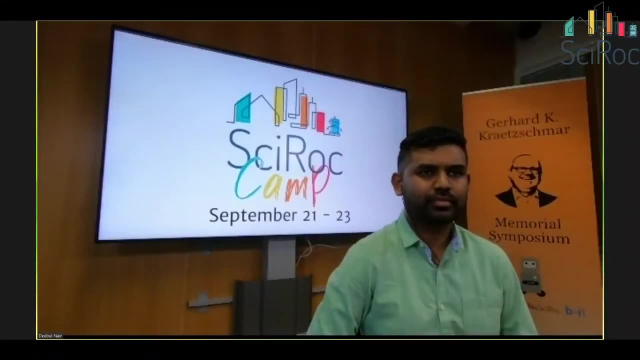 Hello everyone and welcome to the skyrock camp. My name is Divul Nair and I will be your host and moderator. Today is the second day of our camp and which is a week-long camp we have planned for you, So the skyrock camp. 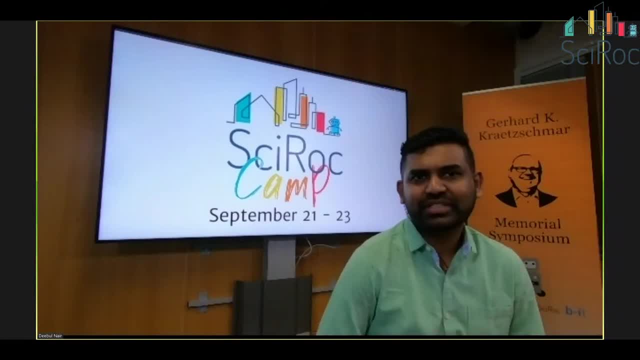 is basically an effort and a skyrock project to train new teams to participate in different robotics competition and different benchmarking, like basically skyrock and robocop and the european robotics league. So yesterday we had a very good session. We had two teams, two teams in the champions talk. 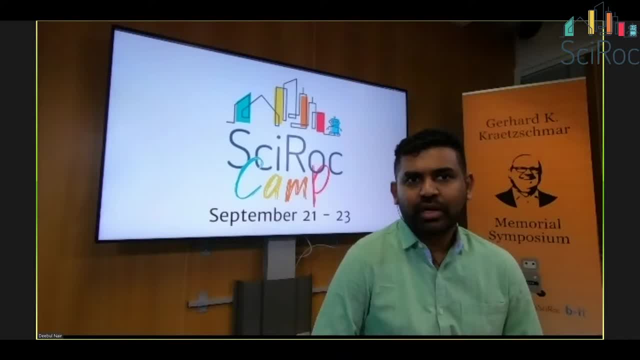 Today. this was very nice in terms of understanding what you call. how do teams perform, what are they thinking, how do they participate, and it was really nice to know from the team's perspective. Today we shift on towards the learning side, But today we have our first 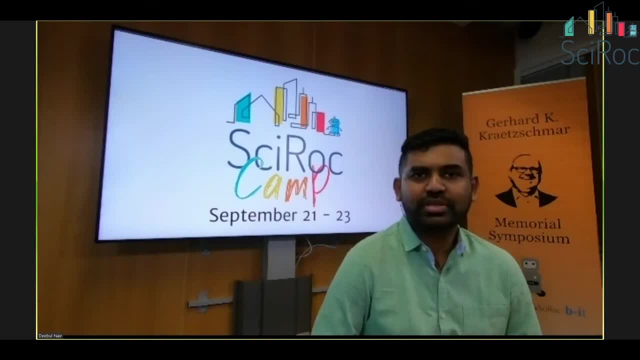 tutorial, and the tutorial is on robot: perception from robotics. Our speaker for today is Mohamad Brazil, Mohamad Brazil. He has a bachelor's in computer science from the University of Dunajoyo Madura, Indonesia, After which he joined the master's program of autonomous systems Hochschiller-Bondainzi. 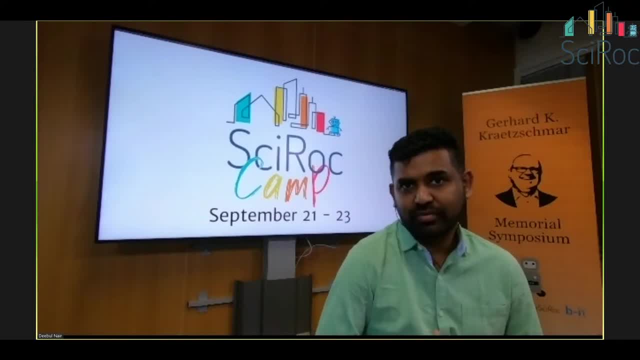 He's an active member of the Bitbots team and, as you might have seen, yesterday we had introduced to the. we got introduced to the Dot's team for the world championship And he contributes towards perception in there. He has participated in different robotics competitions- in robocop and rockin' and rocku2 and european. 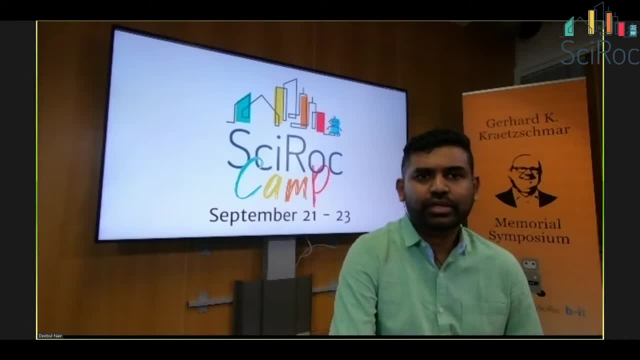 robotics, So he's got a good experience with competition and benchmarking. He also contributes to many open source libraries. He was part of the team which won the world championship in 2019, which is the current world champion in the robocop at work. 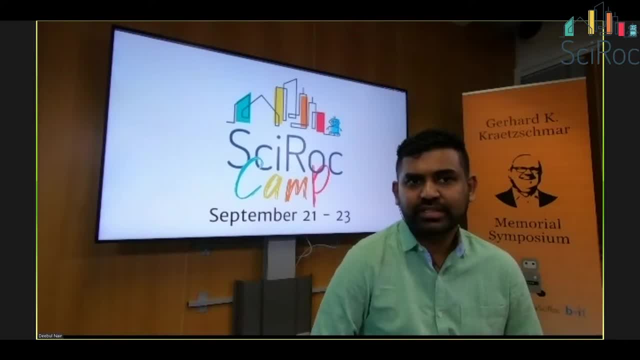 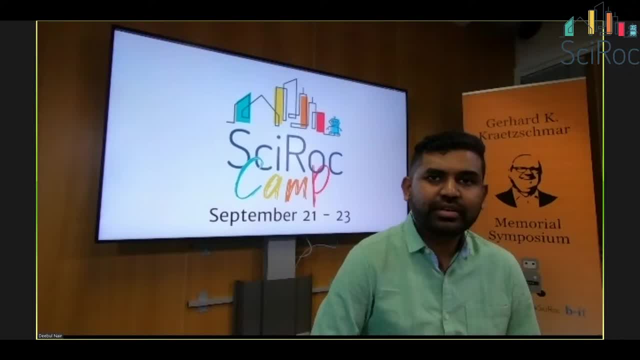 using RGB. I think that's changing of violence, of the image in robotics in general. So I think it's very good to know what this tutorial will have towards this. So today he's giving the tutorial in the perception for robotics. Now he was kind enough to provide us with the video. he recorded it. 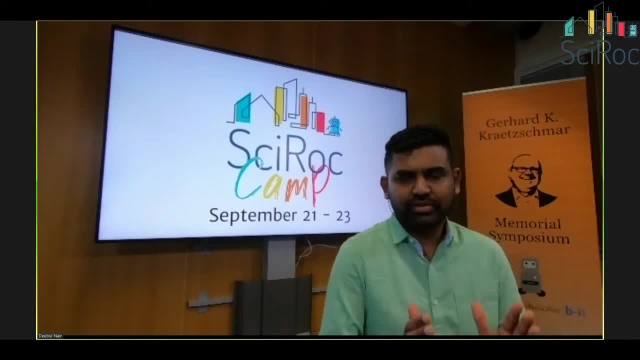 But so we will. we will watch that, but the format is this way. So currently now we will watch him on the video, We will. after the video, I will be joined in live, live by Bazeer and we can ask questions to him from his talk, from the tutorial also the tutorial. 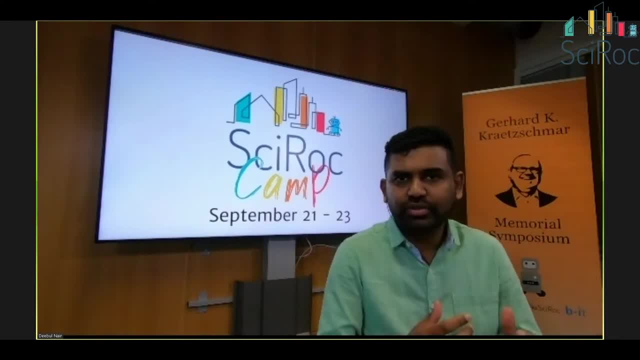 is in a is in a hands-on way. in the end he goes on with sharing you many, many office. it's available in open source, available in github, so anyone can download this and test on their machines. so it's very good for anyone who wants to get it started. also, it's a hands-on kind of a tutorial. 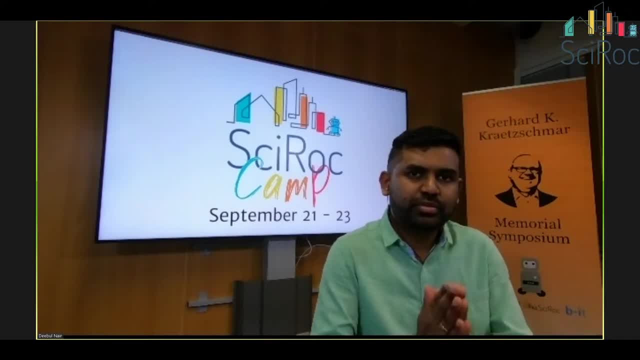 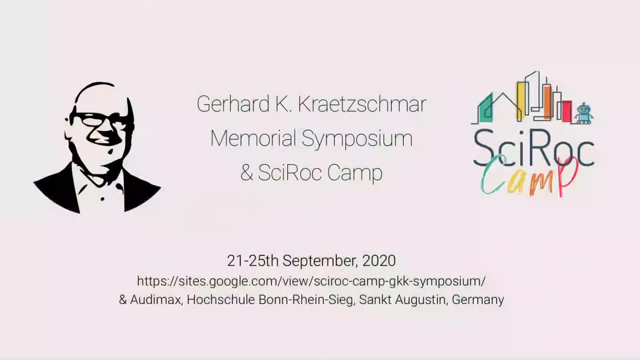 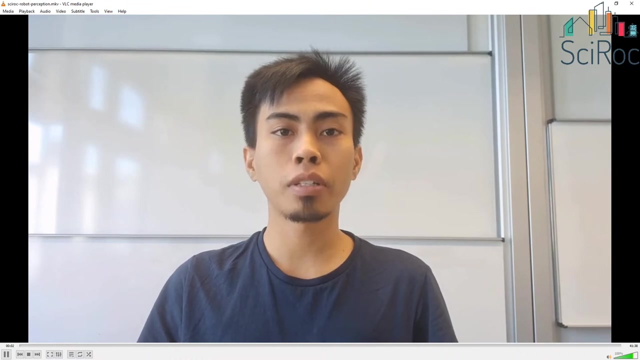 and anyone who wants to ask the questions. please do use the youtube comment sections. we can have it in there. so that's it from me today. so the stage is set now for Wazeel. so, Wazeel, it's up to you. hello everyone, welcome to my presentation on robot perception. i am Mohamad Wazeel. i am a research. 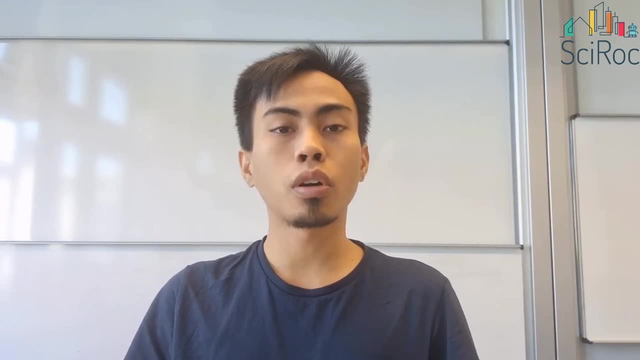 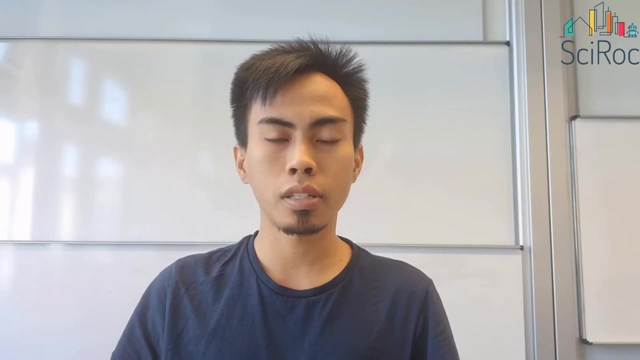 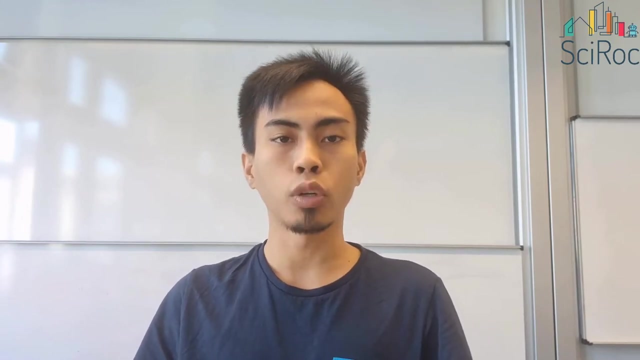 associate at Horseshoe Lab on Rhein-Zick. my research focuses on robot perception, mainly on 3d robot perception. i have been to several robotic competitions, such as RoboCup and European Robotic League since 2017, and in bitbot i am an active member, maintainer and contributor of our 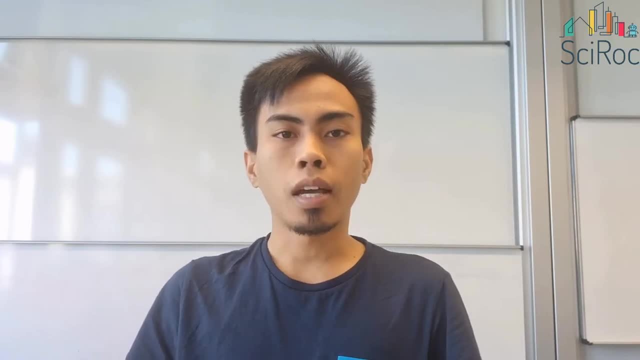 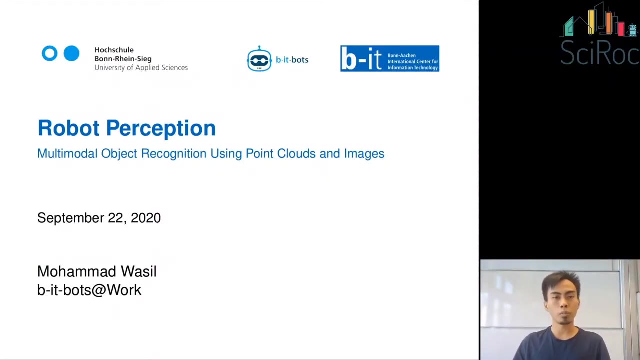 open source industrial robotic software. i work mostly on robot perception and now i will present our approach on multi-modal object recognition using point clouds and images. in this talk we will mostly focus on the perception of robot, which mostly operate on industrial environment and smart city environment. let's first take a look at the environment and the 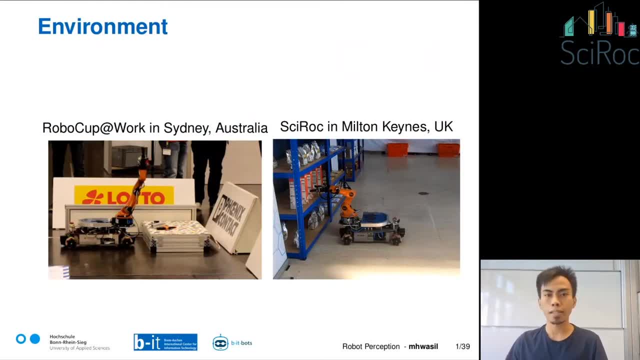 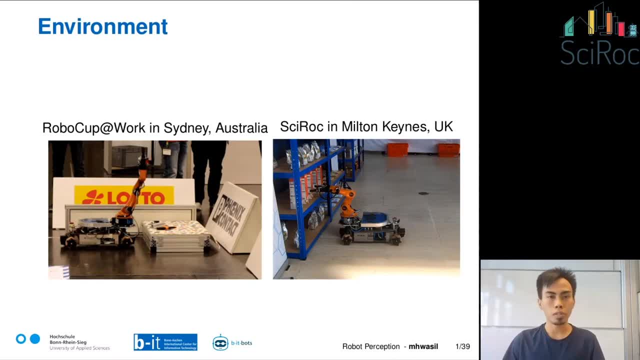 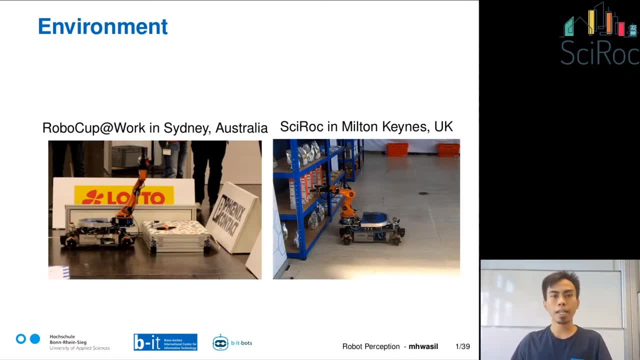 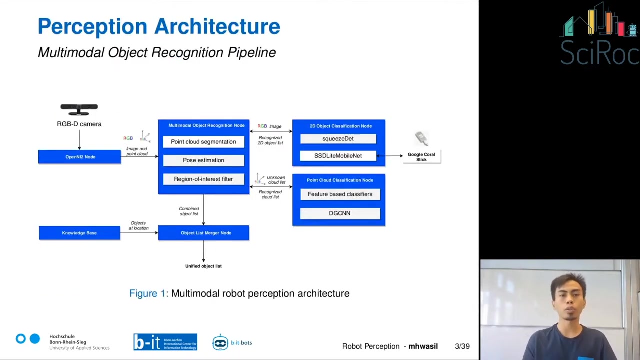 and the camera look forward instead of face down and there can be decoy or fake objects on the workstation and those objects have to be avoided by the robot. let's begin with our perception: architecture, architecture: in here we have rgbd camera and open ni node on the left side. 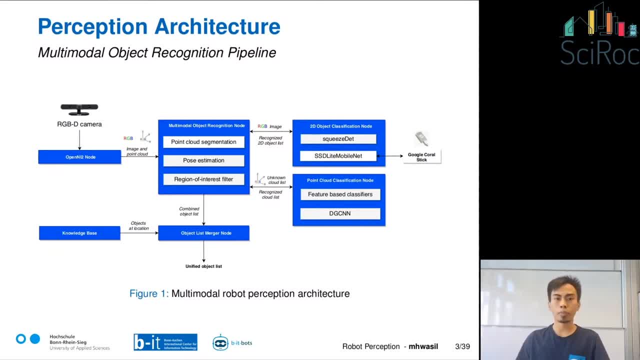 open ni node has success to the camera data and then from this open ni node the image and point clouds is published to a ROS topic and then multimodal object recognition node subscribe to that topic using ROS message filter, such that we have the same object from the same timestamp, since here we have two topics which, and thus we 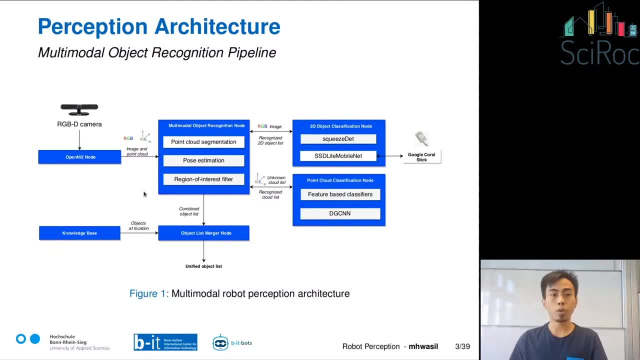 need to synchronize them. we start with the point cloud segmentation by separating the points above the table and the table. once we get the image and the point cloud, we first segment the point clouds to separate the tabletop objects from the table and we use run sucks to do this, and this is done via pcr library. 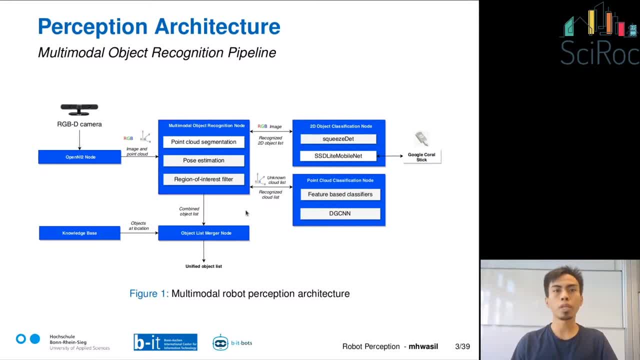 then once we get, once we segment the point clouds, we send the image to the 2d object classification node and then send the tabletop clusters to the 3d object recognition node. as you can see here on the right side, we have a 2d object classification node and 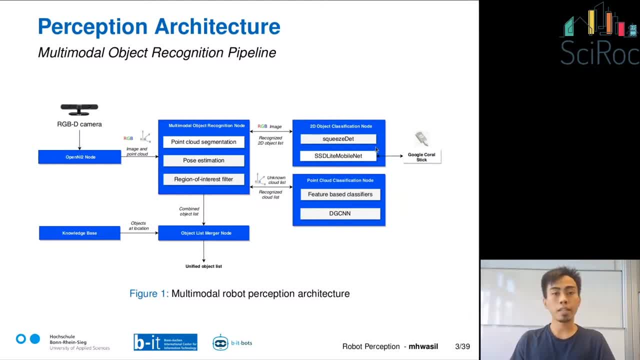 in there. we have two models which are squished debt and SSD lite mobile net. we perform inference on CPU with squished, where we use stipu to infer the image. if we use SSD white mobile net delle. Both models are a single object detection and classification which output bounding boxes and class probabilities. 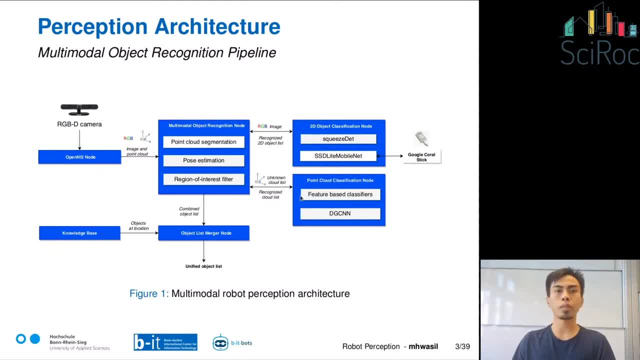 And then next, to classify the point clouds, we have two different methods. One is a feature-based method with SPM and random forest as classifiers, And then we also have a deep learning method using a graph convolution. Once we get the object recognized from two modalities, then we estimate the pose from both modalities. 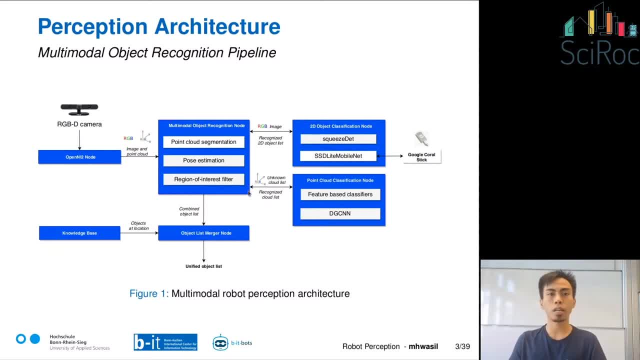 And then we filter out some objects which are out of interest. For example, if we are only interested in the objects on the table, then we filter out the objects which are not on the table, And it is useful if we have different environments. 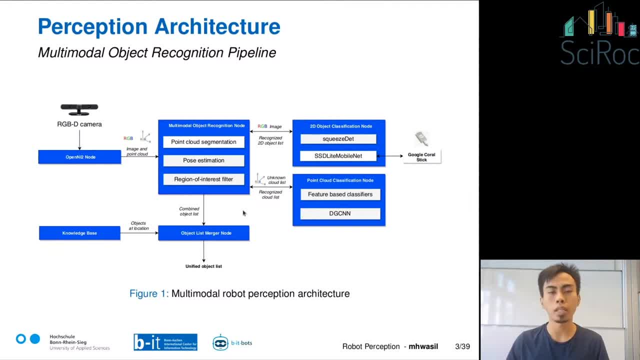 For example, if we have a smaller table, then we can filter out the objects which are not on the table And then we can also update the region of interest, And this can be dynamically updated via RQT. Then, once we get the list from both modalities, we publish them to the object-list. mergers. 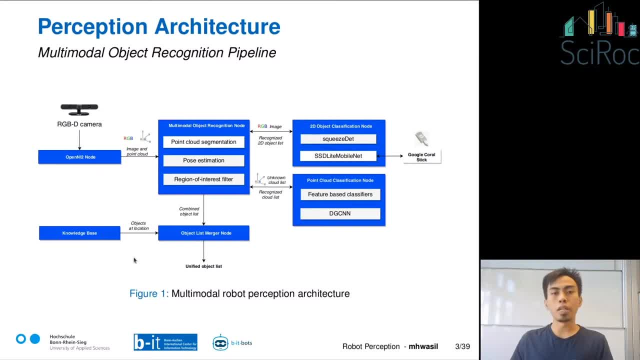 And in the object-list merger, as the name suggests, it merges the two lists based on some criteria which I will explain in the later slides. The object-list merger node also gets some information from the knowledge base about the facts in the location. 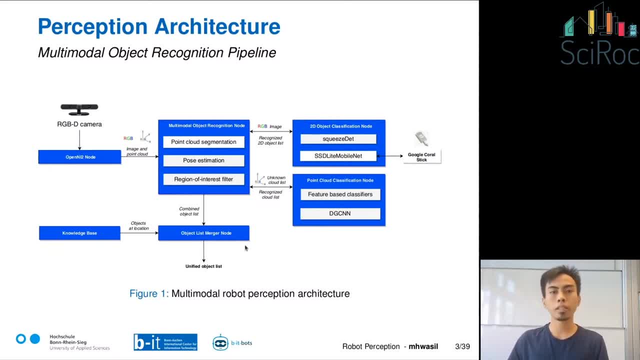 what are the objects on the inventory And then from the object-list merger, it publishes a unified object list. You might be wondering why we use two modalities, why we use 3D and 2D. So let's start with some motivation and the problems that we face during the project. 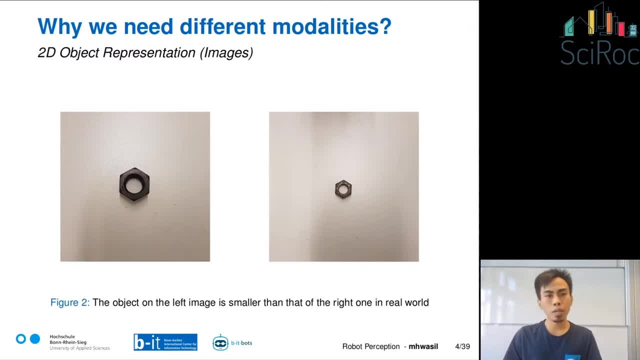 The main problem with the image is that it is a 3D representation of an object, while the object itself is in a 3D world, And thus we lose some geometrical properties of the objects. For example, here on the left we have a picture of a nut. 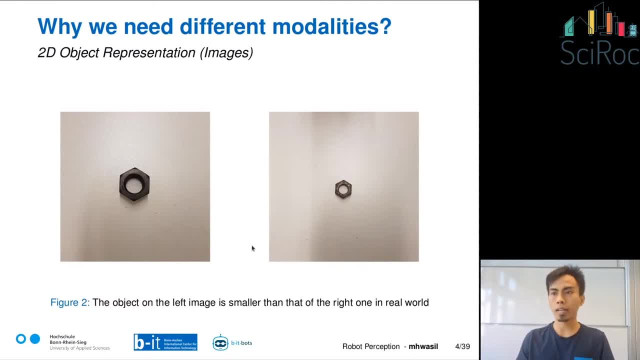 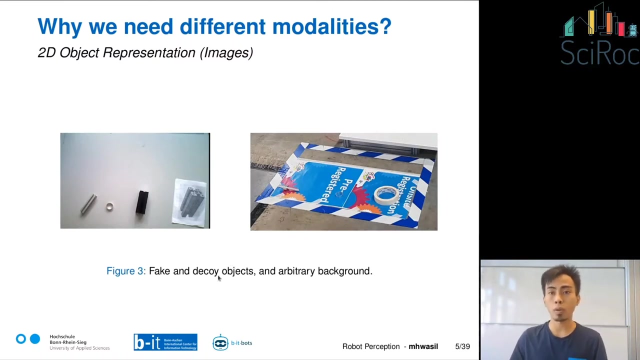 This is actually smaller than the right one, But since the camera position is different, so it seems that the small nut looks bigger on the image plane, while the big nut looks smaller on the image plane. Secondly, deep learning on 2D can be fooled by a picture of the object itself or a fake object. 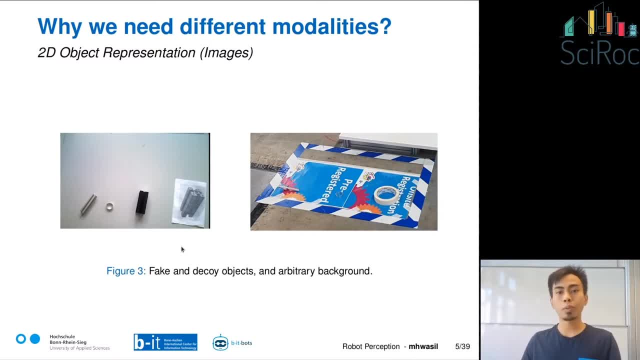 For example, here on the left image, we have two aluminiums. The right aluminium is actually fake. It's just a photograph of the left one, But since they are taken from the 2D camera, they look the same In most of the time. deep learning on 2D will fail on this situation. 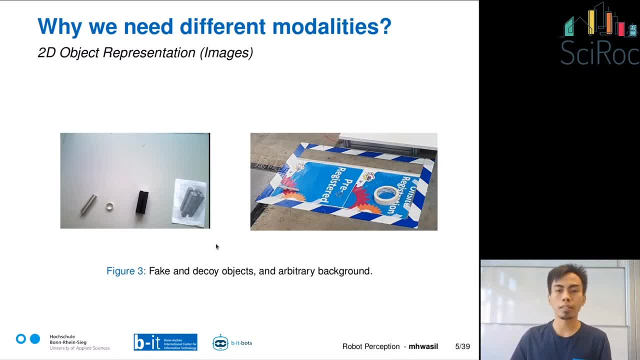 because they don't have any other properties which can differentiate between the real one and the fake one. On the right image, we have an arbitrary surface, meaning that the background of the table can be different And this background can be similar to the colour of the object. 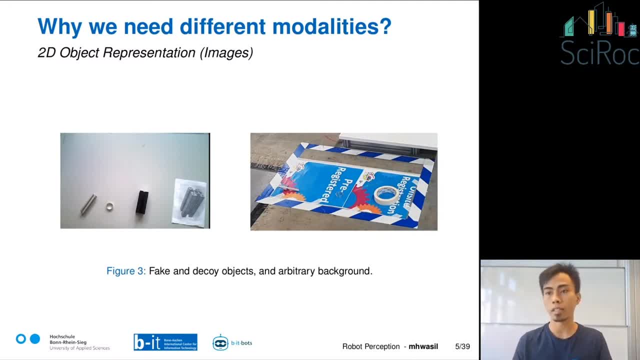 For example, if we have a grey axis in here and the background is also grey, then we cannot see the object clearly using the 2D camera. But on 3D we will get a point representing the axis. It doesn't matter what the colour of the background is. 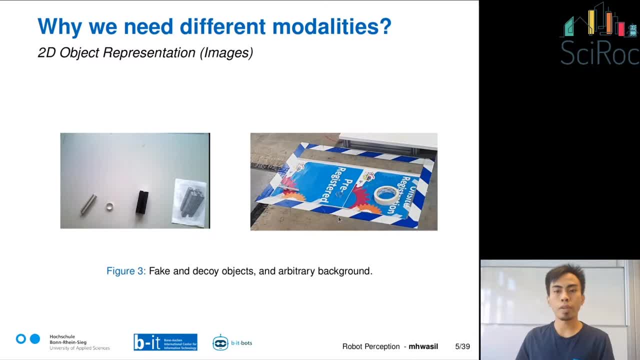 Even though this random or arbitrary surface can be addressed by augmented training, but it is still challenging due to some, for example, similarity between the object and the background, and somehow the camera just cannot see the object. What about 3D representation, then? 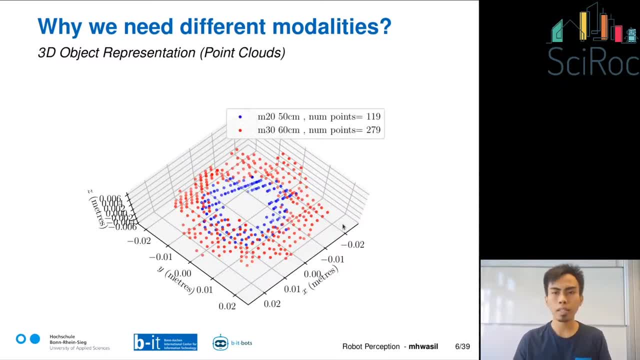 So in this case it is a point cloud. Then, as you can see here on the slide, we have a 3D representation of nuts. The red points represent a big nut taken from a farther camera distance, while the blue dots is a small nut. 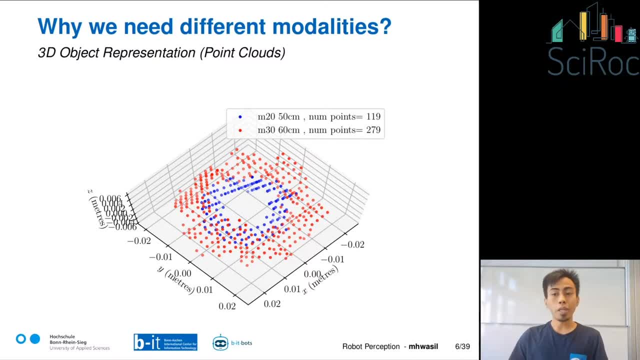 and they are taken from the closer camera distance. If we use 2D then this small nut will look bigger, as you can see in the previous slide, But in here it still preserves the critical points of the nuts. These are the points which make this representation a nut. 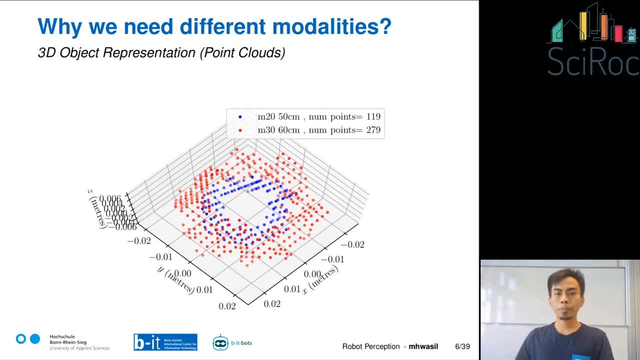 or a big or small nut. So in 3D it doesn't matter if you vary the camera distance. so the shape of the object or the size of the object will still be the same, even though the density might be different, because the closer one might be more dense. 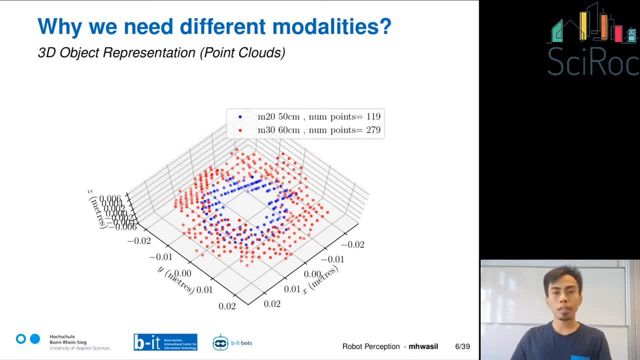 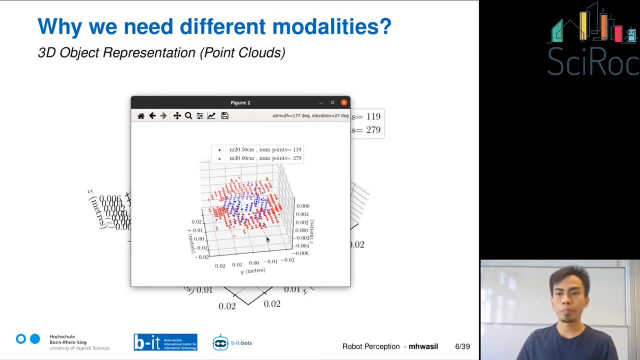 while the farther one might be more sparse. We can take a look at the 3D plot of these representations. As you can see, here we have the same small and a big nut. They still represent its original size and the size is the same as the one in the real world. 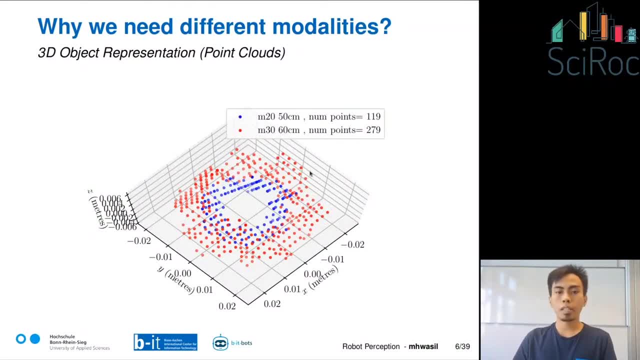 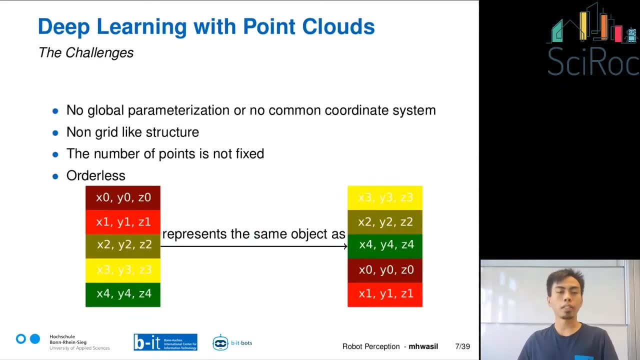 Nonetheless, deep learning in 3D does come with some challenges. Unlike images, point clouds do not have global parameterization or there is no common coordinate system, And it is a non-grid-like structure. like image, it is just a matrix of pixels. 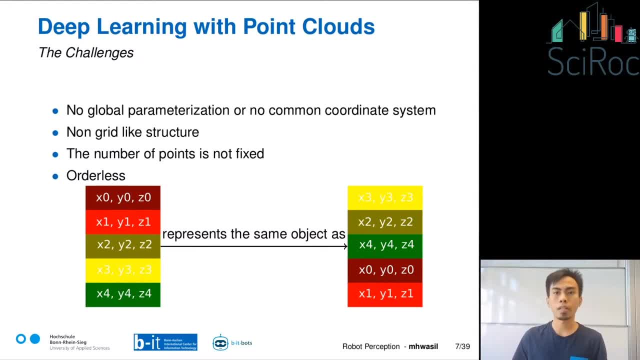 And then it has a variation in the number of points, so meaning that the same object can be represented by a different number of points. And, lastly, the point clouds are orderless, meaning that the position of each point can be scrambled, but they can still represent the same. 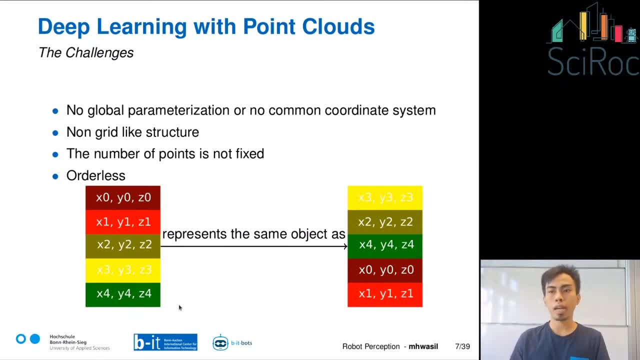 As you can see here on the slide, we scramble, we move point 0 to the number 4, and then number 4 to the number 3, but they can still represent the same object. So the challenge here is that it is invariant to permutation. 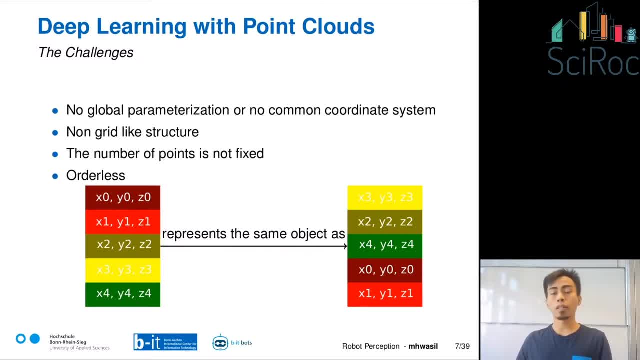 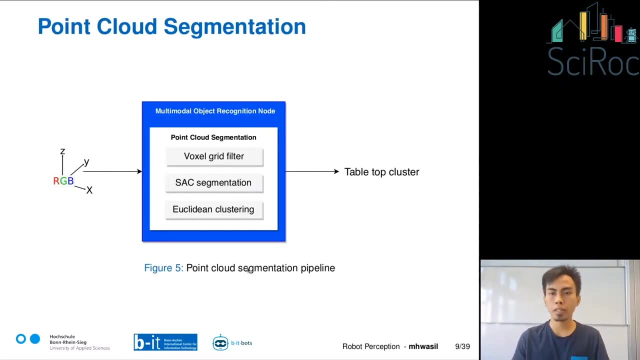 meaning that if you multiply this by the weights- different position of the points- they should result in the same object. Let's continue with the point cloud segmentation. On this slide we have a point cloud which has color and then a multimodal object recognition node subscribes to that topic. 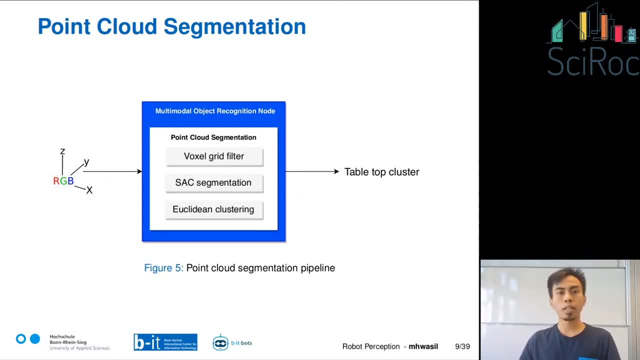 to the point cloud and then, once it gets the point cloud, it filters out the points, because we want to reduce the number of points and thus reduce the number of computations. And then we apply sag segmentation and then, once we get the plane equations, 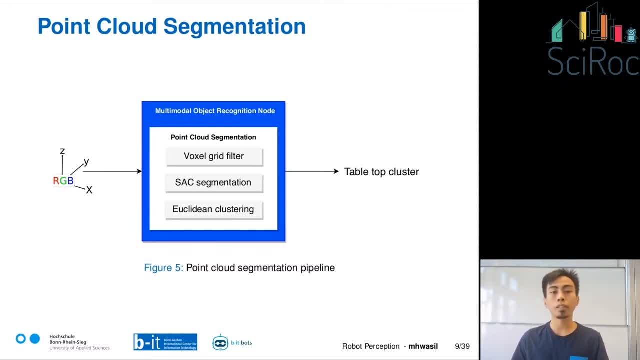 we fit a polygon and then we take the points above that polygon and apply clustering using Euclidean distance, and each cluster represents one point cloud or one object on the table. So, as you can see here on the left image, we have a raw point cloud. 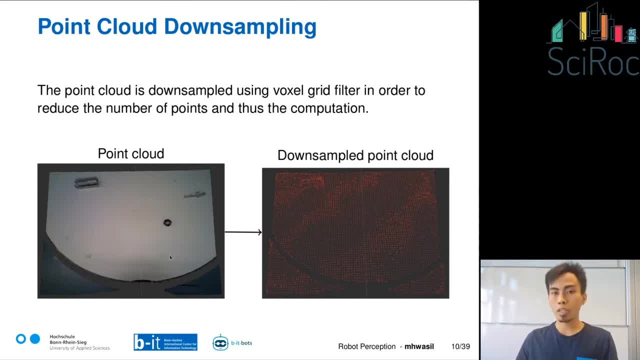 which has a very dense point. I think it has more than 300,000 points- and then we downsample them here on the right side we have with the red color, and they are more sparse than the original or the raw point clouds. 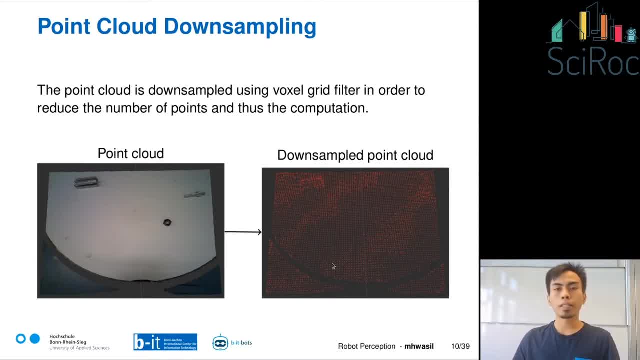 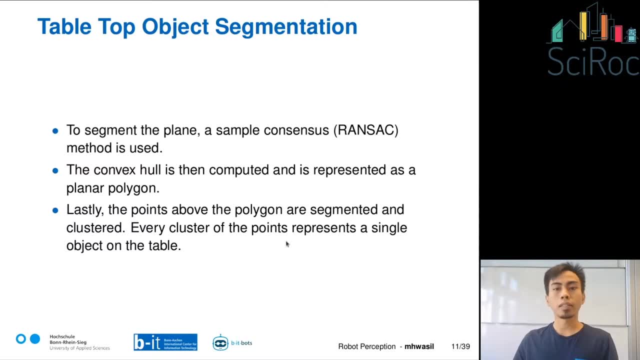 And then, after the voxel grid filter, we segment the plane, find the equation using RANSAC, and this is done via PCL library, and then we apply a convex hull and then also compute the polygon, the planar polygon, and then, lastly, 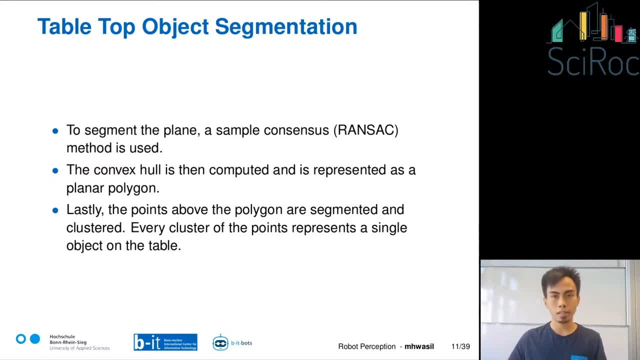 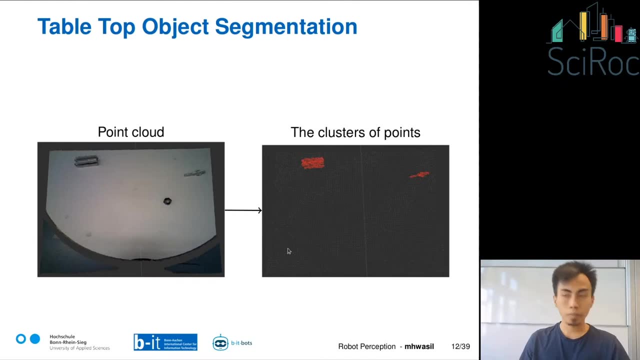 and we take the points above the polygon and cluster them, and each cluster of the points represents a single object. on the table, As you can see, here we have a raw point cloud and then filtered by a voxel grid filter and then the red points is a cluster of the objects. 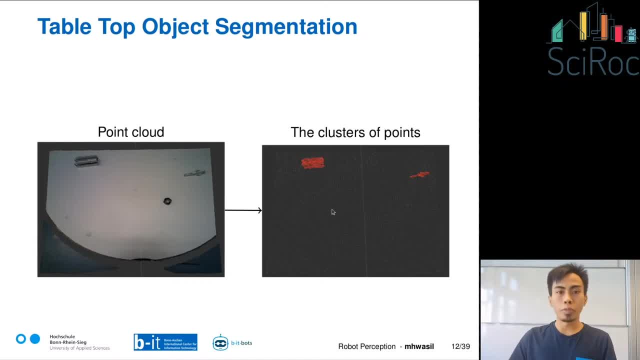 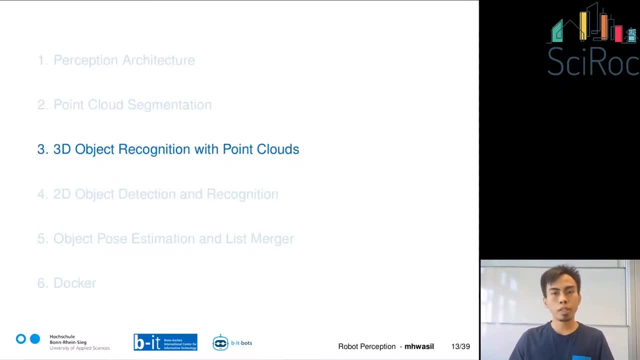 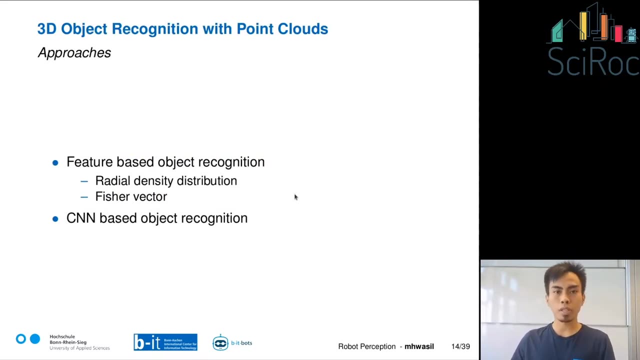 Once we get the clusters, we send these clusters to the 3D object recognition node to be recognized. Let's continue with the 3D object recognition node with the point clouds. So we have multiple approaches here. We have feature-based approaches. 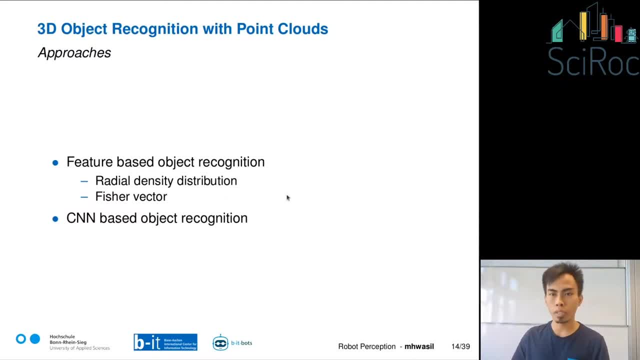 and in these feature-based approaches we combine two features. One feature is coming from radial density distribution and then the second one is a Fisher factor, And lastly, we have a CNN-based object recognition using dynamic graph convolution. These two different methods come with advantages and disadvantages. 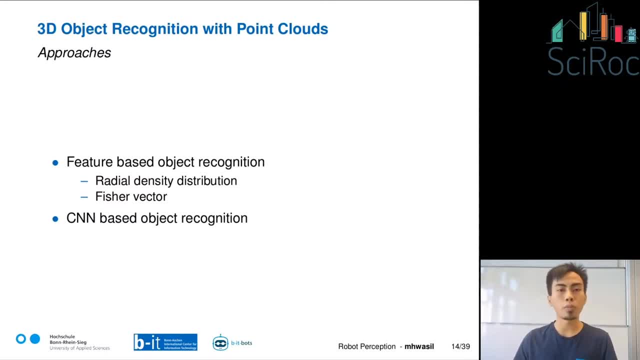 For example, feature-based object recognition can be trained faster, so if we have a new challenge and we have a new object, we can just collect the dataset and then train them in less than 10 minutes, While the CNN-based classification method is more robust. 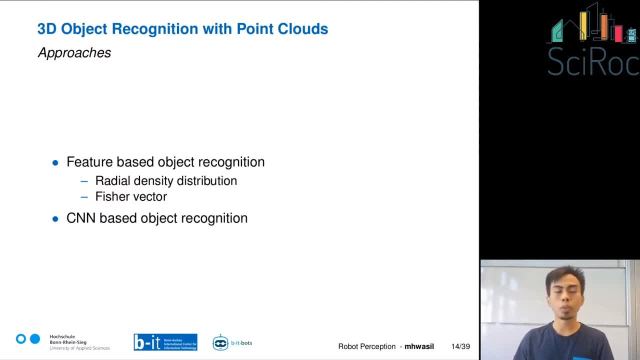 however, they are tied to a particular object. So if we have new objects then we need to retrain them and then the training will take a lot of time. So during the competition, if we have new challenge, new objects, it is better to use a feature-based object recognition. 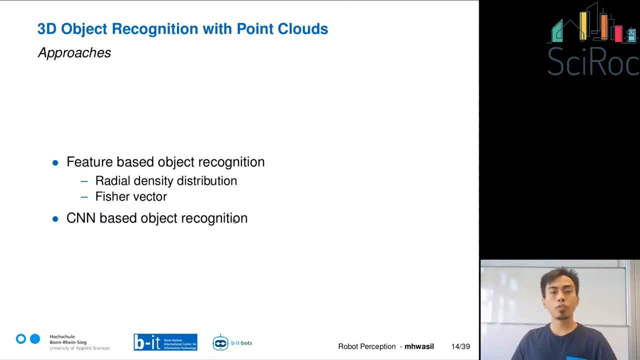 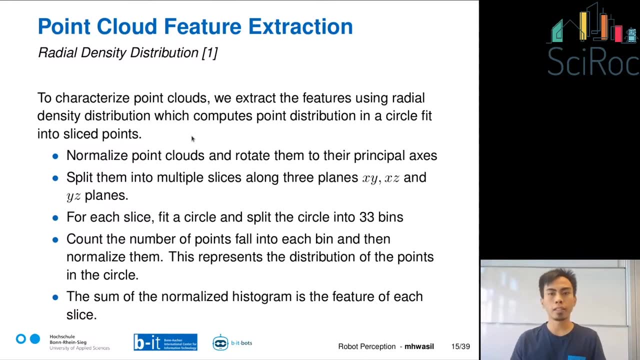 because we can train them faster. Let's begin with the feature-based point cloud feature extraction. We start with radial density distributions, So the idea here is to slice the point clouds along three axes- XY, XZ and YZ planes, And then, for each slice, 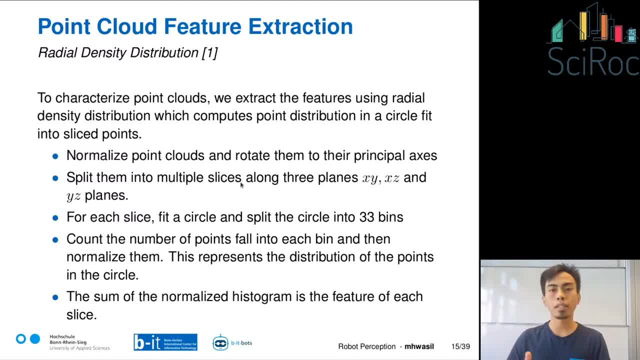 we fit a circle and then we divide the circle into 33 bins, So the points which fall into each bin are calculated and then sum, And the sum of this histogram is the feature of each slice. For example in here on the left: 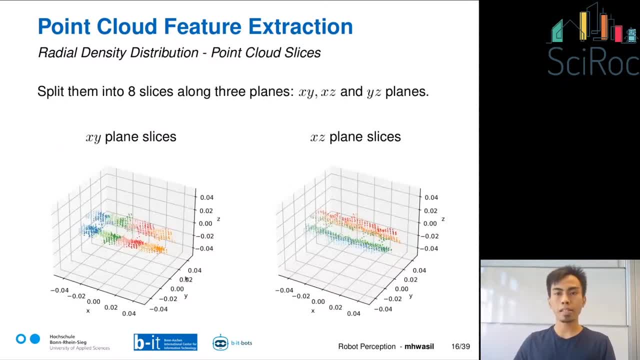 we have a XY plane slices and the color represent each slice, While on the right side we have a XZ plane slices And it's the same: the color represents one slice along XZ plane. This method is actually an extension of our approach. 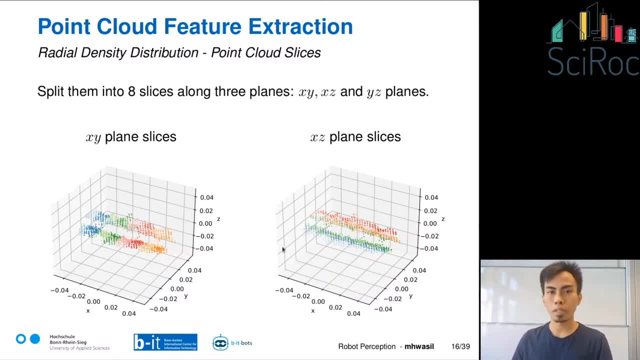 which was presented by Santos in 2017.. And it was using one plane instead of three planes. Let's take a look at the at the circle, at the points in the circle And on the left. here we have a XY planes. 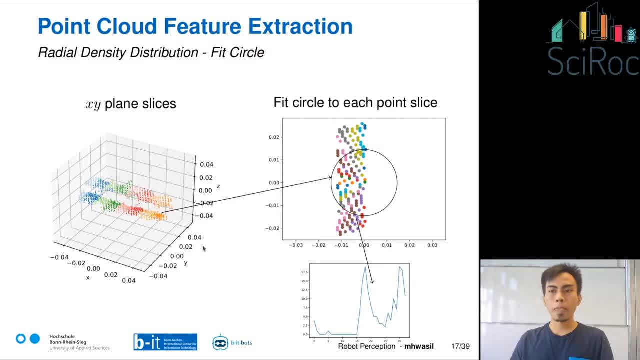 XY plane slices, And then for each slice we fit a circle like on the right image. So in here each color in the circle represents one bin or one one, one area, And then we count the number of points which fall into each bin. 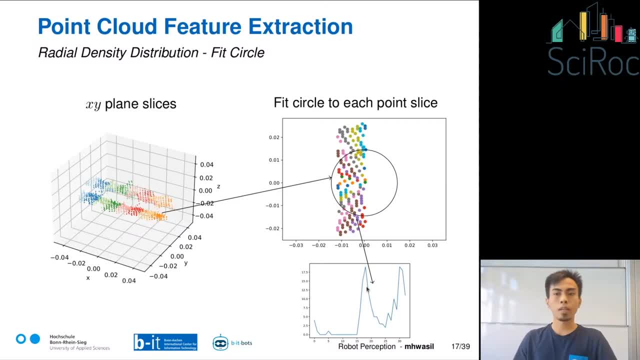 And then we compute the histogram for each circle. So eventually we have: if we have eight slices, we will have eight features. Since we have three planes, then we would have eight by three features, which is 24 features, Moving on to the Fisher vector feature. 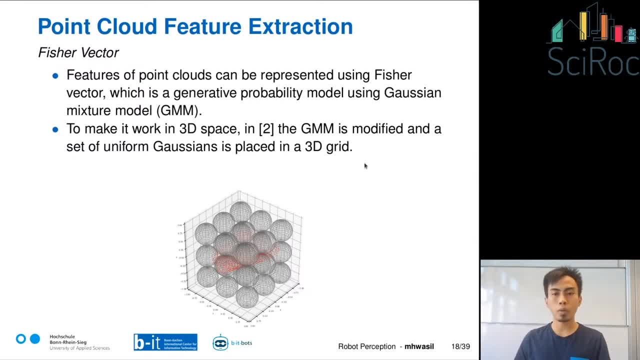 it is actually a generative model which is derived from Gaussian mixture model And it was used to classify images And this was one of the of the state of the art before the deep learning era. To make this work on a point cloud, 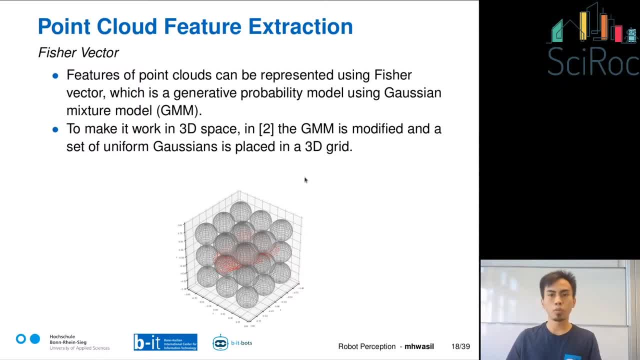 So in this paper the GMM is modified and a set of uniform Gaussians is used And they are placed in a 3D grid Like in the picture. in here we have a three by three by three Gaussians, So meaning we have 27 Gaussians. 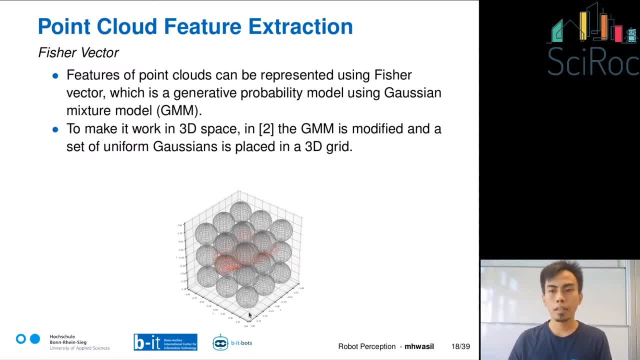 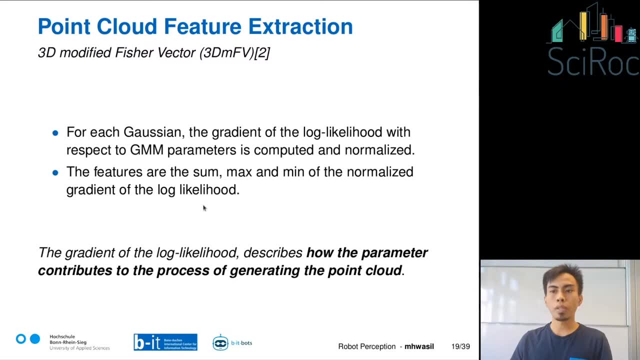 And then what are the features? Let's move on to the next slide. So for each Gaussian in here, for each Gaussian, we compute the gradient of the log likelihood with respect to each GMM parameters, And then we normalize them. The features are the sum. 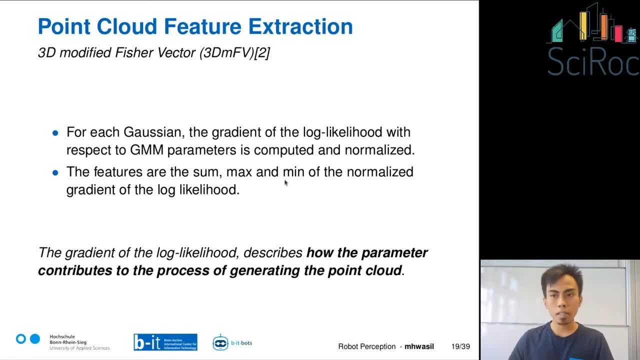 the sum of the parameters and the max and the min of the normalized gradient log likelihood. So what does this normalized gradient likelihood tell us? This gradient describes how a parameter of each Gaussian mixture model contributes to the process of generating point clouds. So meaning, if there is no point inside the Gaussian 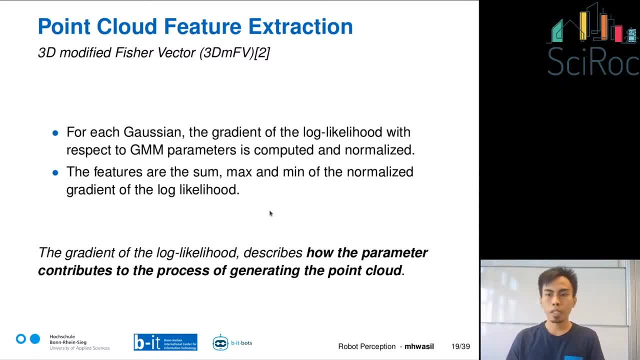 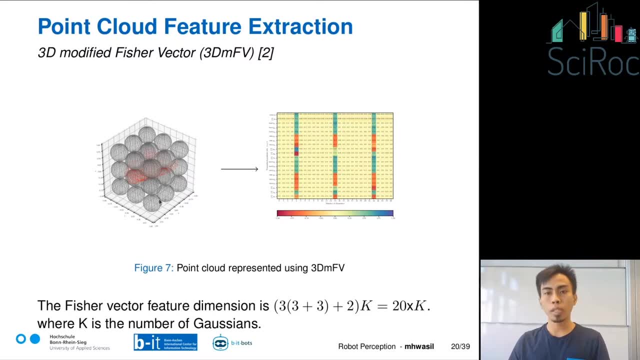 then it does not contribute, It will be zero. And then let's take a look at the feature representation using Fisher vectors. On the left side, we have 27 Gaussians, And then on the right side, we have the features, which is nothing. 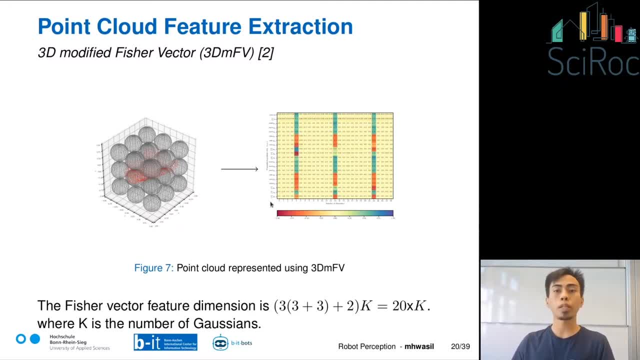 but the gradient of the log likelihood with respect to the GMM parameters. In here we have 20 by k features. Why not 21?? Because we only take the sum, the sum with respect to each Gaussian parameter, meaning that we would have the weight of each Gaussian. 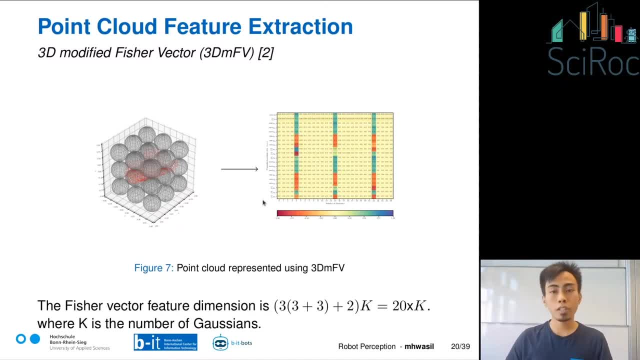 And then we have the mu and then sigma, And then, since it is 3D they are, the weight is 1, and mu is 3, and then the sigma sigma is also 3.. We did not take the weight of the Gaussian mixture model. 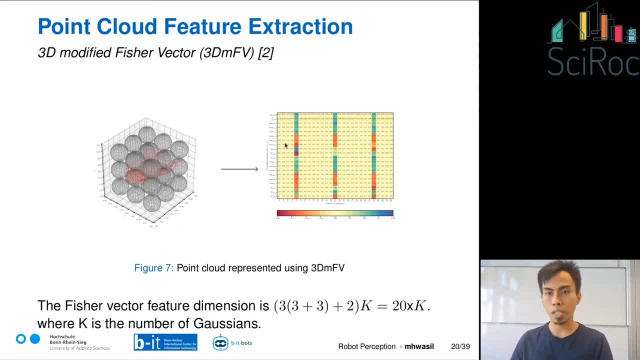 because the weight corresponds to the farthest point, sampling, meaning that it is always zero. That's why we have 20 by k instead of 21 by k. So what does this feature tells us For each row? it is actually the parameters of each Gaussian. 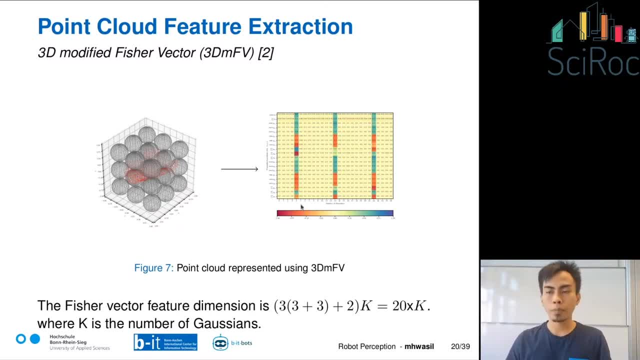 And, as you can see here, the only three Gaussians has variation in the number, while the rest are zero, meaning that there is no point in the, there is no point in the Gaussian, Once we get the features from both RTD and 3D MFE. 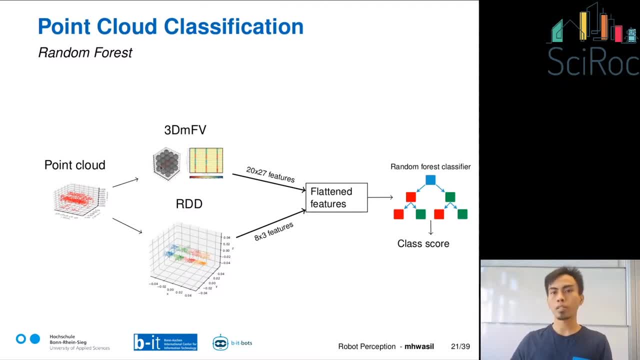 we combine them. As you can see here on the picture, we have a point clouds and then 3D MFE on the top and then radial density on the top And then radial density distribution on the bottom. So we have 20 by 27 from 3D MFE. 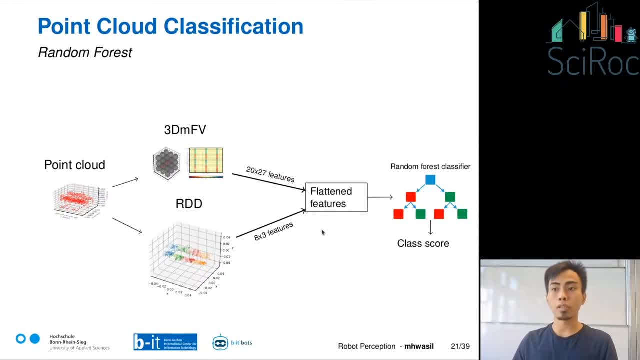 and then 8 by 3 features from radial density distribution And then we fed them as a input of the random forest classifier. This can actually be trained using deep learning or other methods like SVM, And why we combine them? We did some evaluation on this. feature extraction methods. 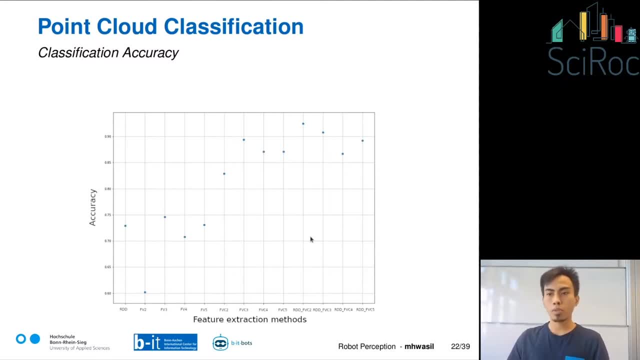 using a random forest classifier And, as you can see here on the plot on the very left, we have a radial density distribution. This was tested using our industrial data sets. And then we have a Fisher vector which has different Gaussian, for example 2,, 3,, 4, and 5.. 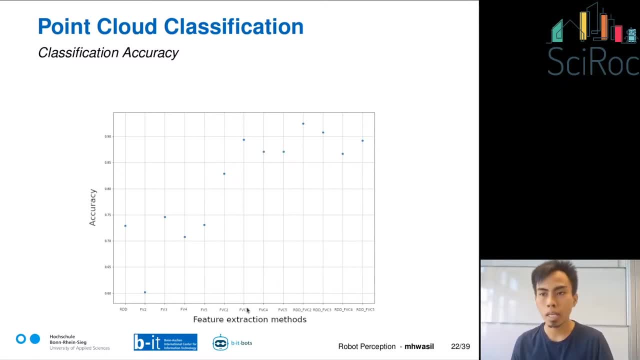 2, meaning that we have 2 by 2 by 2, meaning we have 8 Gaussians. And then we have a combination of the Fisher vector plus the color, because the color is also RGB. we have 3 points, so we treat them as a point as well. 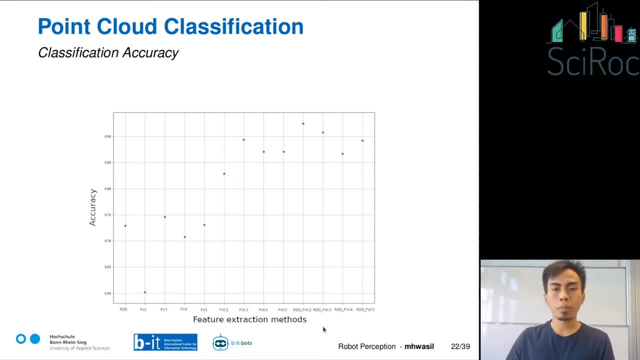 And then we have a combination between radial density distribution and Fisher vector plus color. As you can see here, the radial density, the combination of radial density and Fisher vector plus color, has a better accuracy compared to other methods. Let's move on to the point: cloud classification using deep learning. 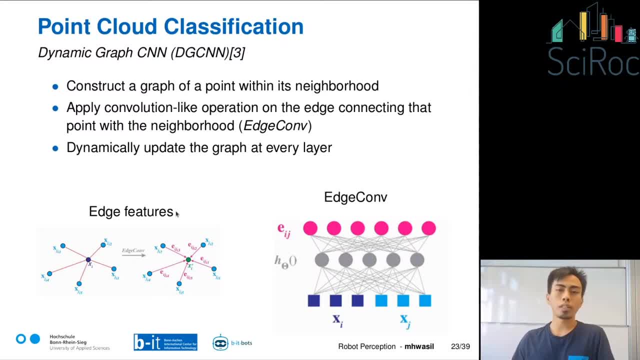 In this case we use dynamic graph convolution. So how does this work? For every point, we construct a neighborhood and then compute the ages, And then we apply convolution-like- or this is just an MLP- to the ages connecting that point to the neighborhoods. 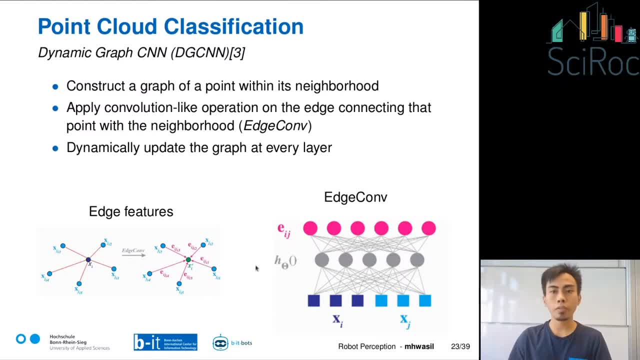 And then for each layer the graph is updated and therefore it is called dynamic graph convolution. It is an end-to-end learning which takes point clouds as input and then output the class score. However, we made some modification in here. 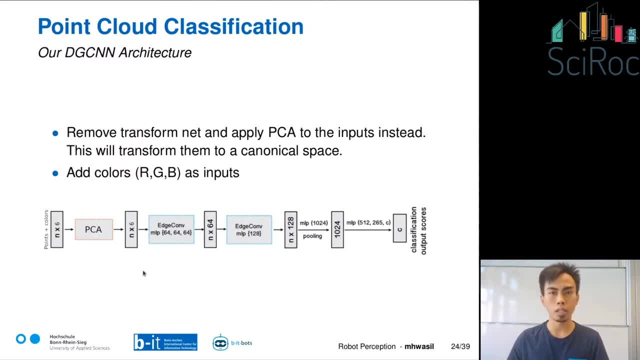 For example, we removed the transformation network because we don't need it. This transformation network is similar to what? similar to the one in point net. This actually transformed the point cloud into a canonical space. Since we normalize the point cloud, we don't need this transformation. 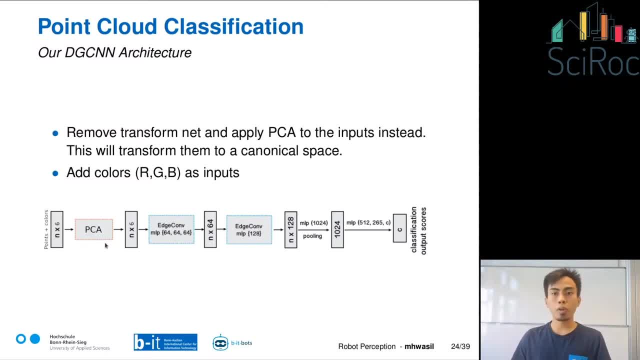 And we also found out that it performs similar with and without transformation, but it is obviously faster without this transformation network. And then we also add color Instead of just 3D points. we have 60 points in here, Because in our environment 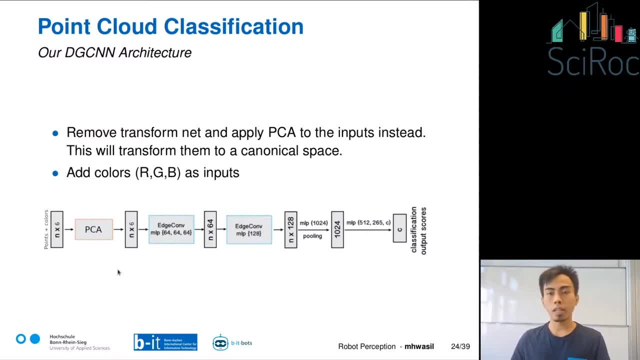 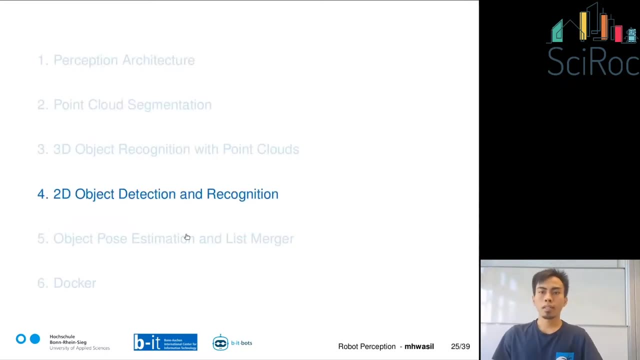 we have two objects which has the same shape, but they are different in color. Yeah, that's it from the point. cloud classifications. Let's move on to the object, the 2D object detection and classification. Let's start with the SqueezeDat. 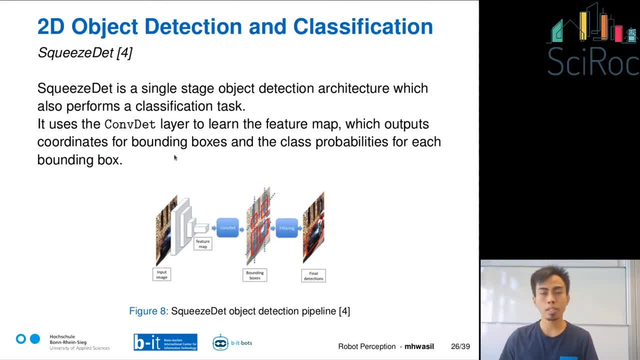 The SqueezeDat is the same as YOLO. It's a single-stage object detection and classifications And it uses ConfDat to learn the feature map and it outputs coordinates of the bounding box and the class probabilities for each bounding box. 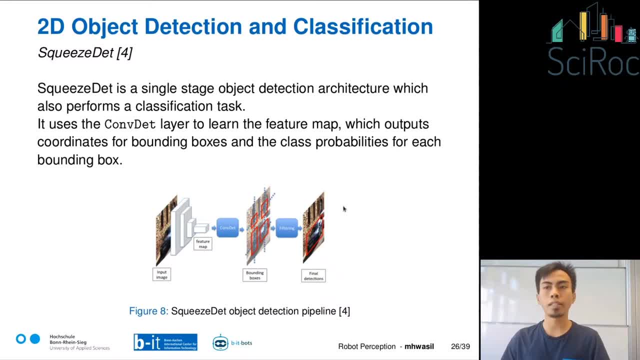 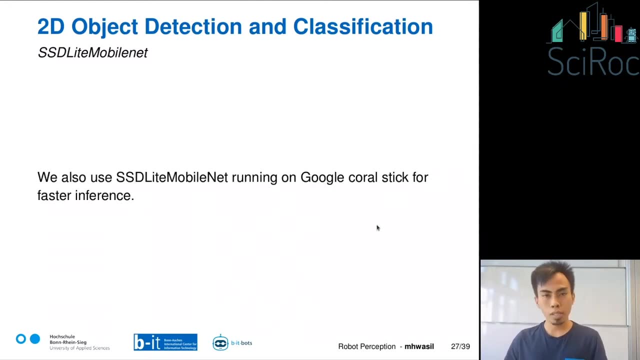 So I'm not gonna explain in detail here what is SqueezeDat and then how does the network look like? We use this as a 2D object detection and classification node, And we also have SSD Lite MobileNet, which uses TPU or Google Coral Stick to perform inference. 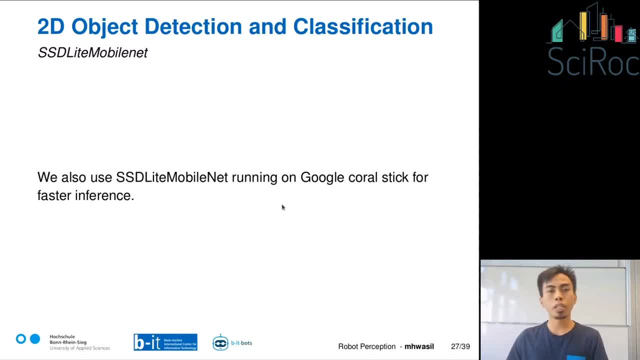 This is actually faster if you do the inference in the TPU instead of CPU. Other than that, we also use Mofidius, for example from Intel, to perform inference on the MobileNet Once we get the objects recognized and localized from the 2D object recognition node. 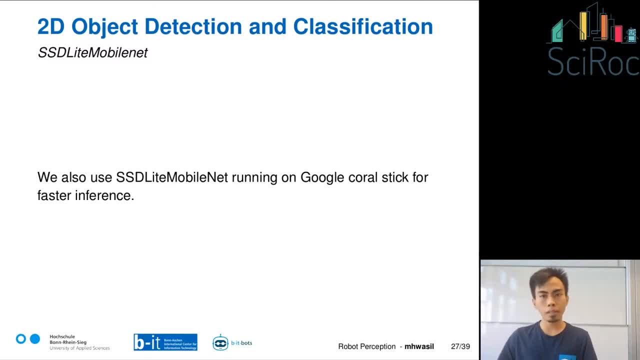 we publish them back to a topic and then the multimodal object recognition node subscribes to that topic. So we only publish the region proposal and the class, probability and the label of the object to the multimodal object recognition node And then 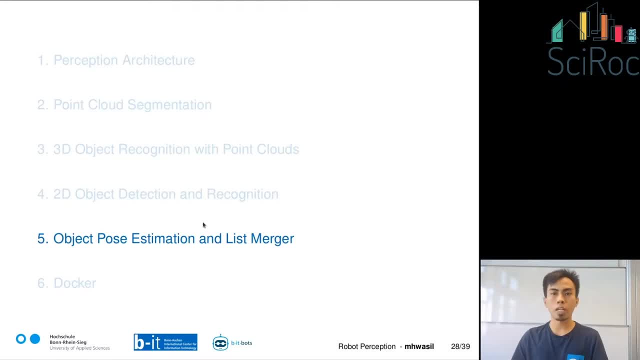 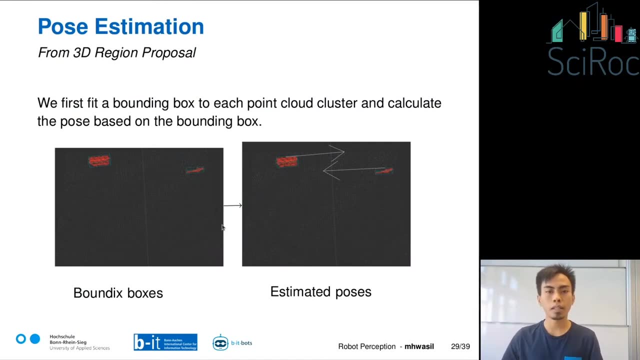 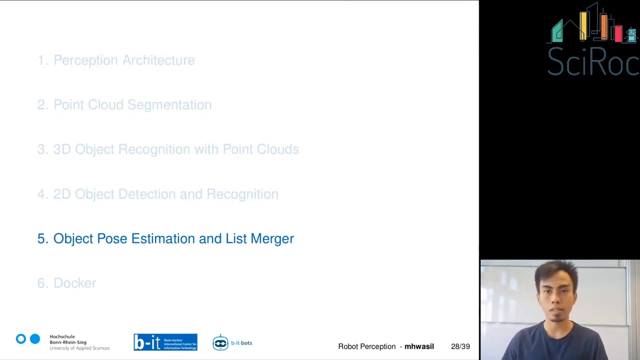 let's move on to the object pose estimation and object list merger. This is where we estimate the pose for each object and we transform them to the baselink and then we merge the object list from the two modalities. Let's begin with the pose estimation from a 3D proposal. 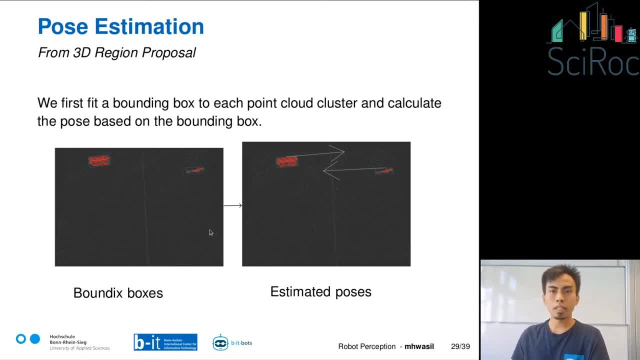 From 3D proposal here means that it is coming from the 3D object recognition nodes and we already have a point class here. so we don't have to find the points in order to get the 3D position. So we fit a bounding box for each cluster. 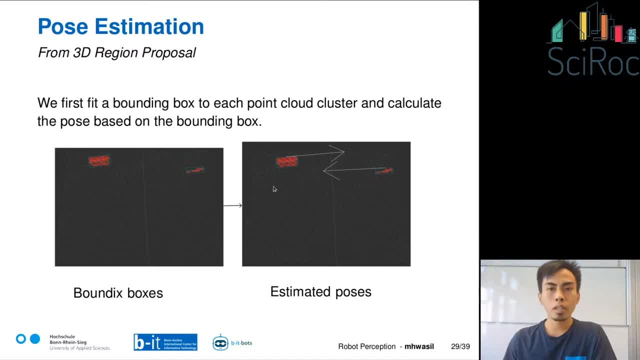 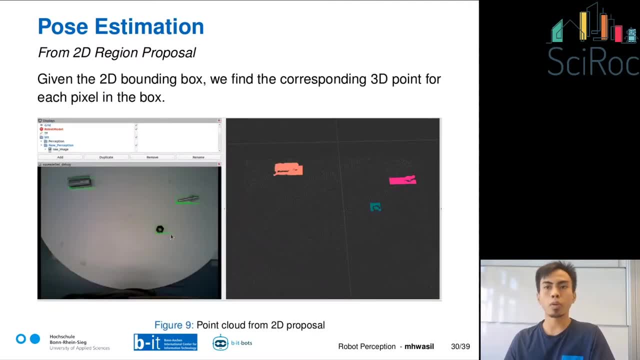 and then find the pose and the orientation based on this bounding box. And then for the 2D proposal, we take the region which we get from the 2D object classification node and then for each pixel in the region, we find the points in the 3D world. 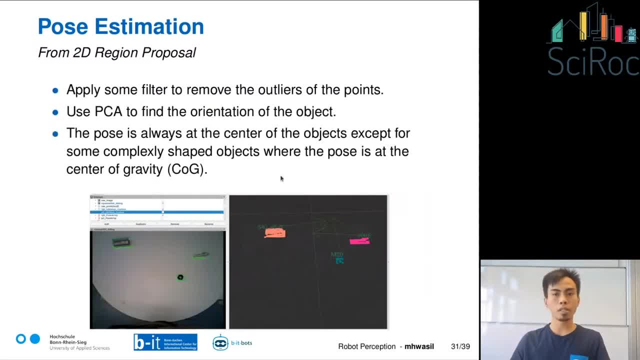 Then, once we get the cluster of the 3D points, first we apply some filter to remove the outliers, For example remove the plane from the object, and then we use PCA to find the orientation of the object. So the pose is always at the center of the object. 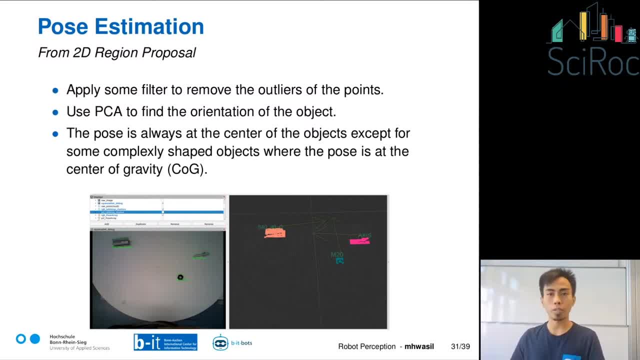 except for some complex points or complexly shaped objects, for example axis and bolt, in which we calculate the pose at the center of the gravity, Such that we can have a successful pick for the robot. Moving on to the object list, merger. 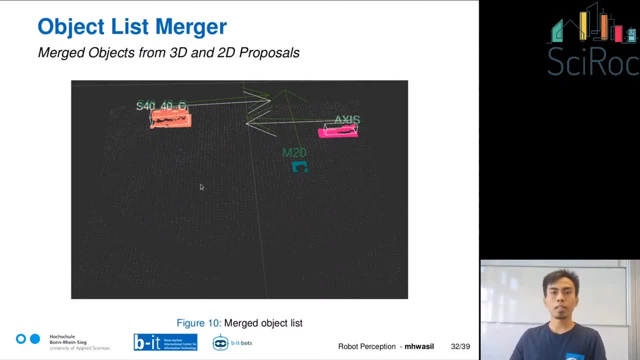 Here. object: list: merger gets two lists: One is from the 3D proposals and then second is from the 2D proposals. As you can see here the white ones are coming from the 3D proposals and then the green ones are coming from the 2D. 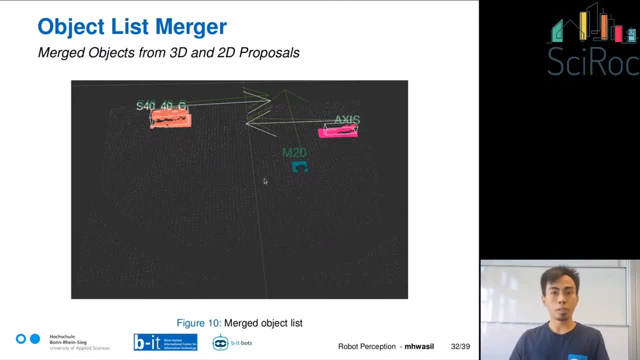 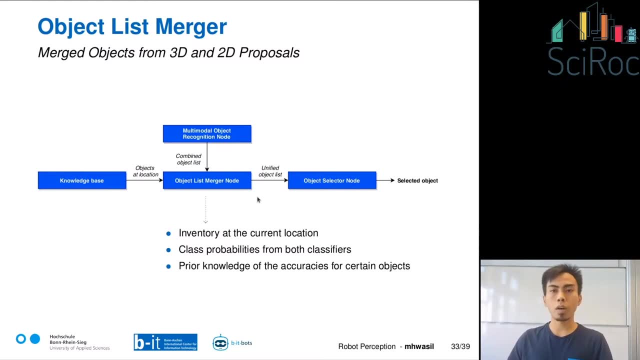 And how do we merge them? So we merge them based on the following criteria: So we have information about what objects are on the table. So this information is coming from the knowledge base which we get from the central factory hub. 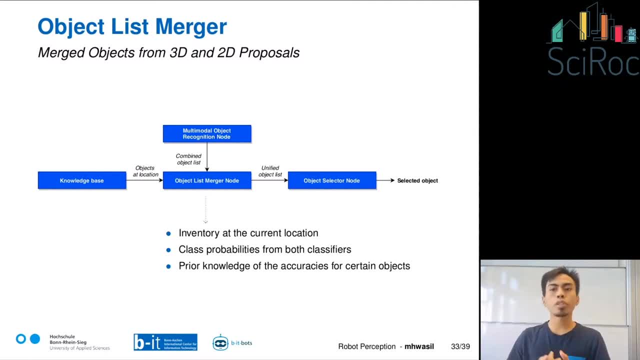 And then we also consider the class probabilities, from what modalities, So which is higher and which is better. And then we also have a prior knowledge about the accuracy for each model and for each specific object, For example if it is about color. 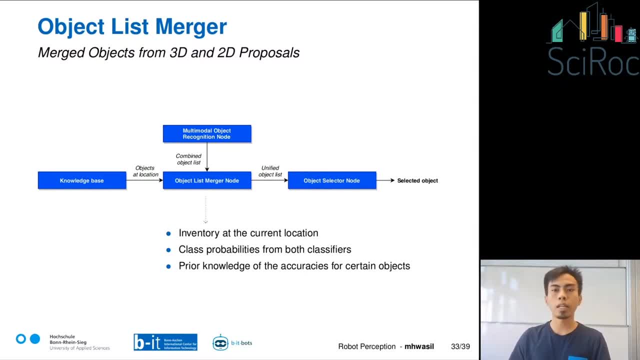 if the model is confused about the color, then we prefer to take RGB, because RGB is always better in color. But if the problem is in the shape, then we take point clouds. We take the proposal from the 3D instead of 2D. 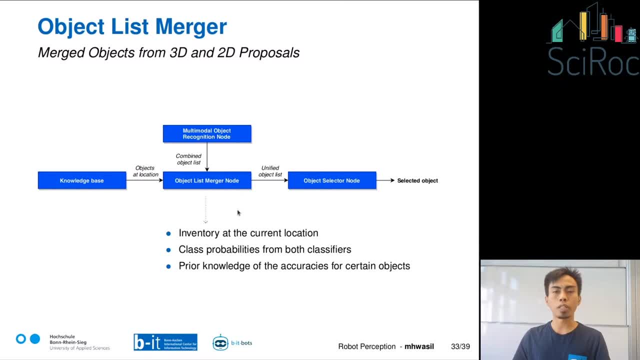 So we combine this thing in the object list mergers and then publish the unified object list to a topic And then object selector node subscribes to that topic. So in this object selector node it does nothing but select objects based on some criteria. 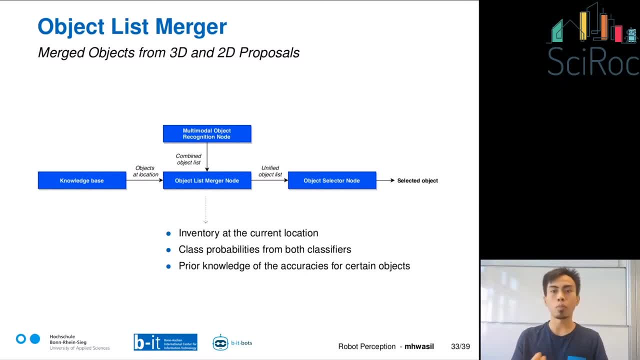 For example, the closest to the robot base, and also we can also pick the objects based alphabetically And then once the object is selected and it publishes this to again ROS topic And then perceived action subscribes to this topic. 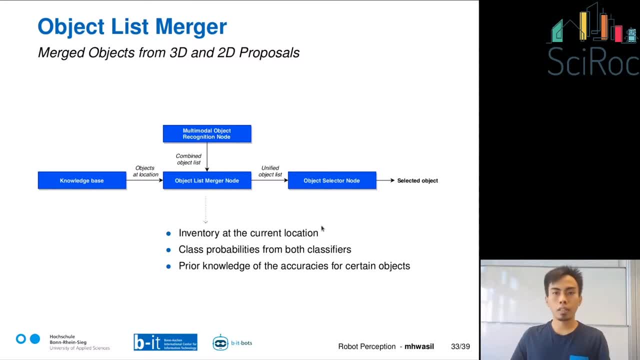 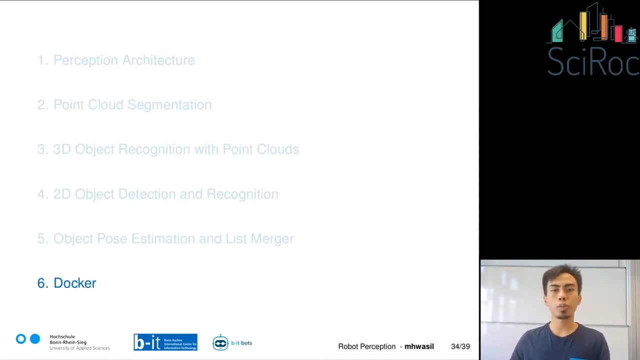 Yeah, that's it for the theoretical part and the architecture. So, to make this presentation less boring, let's do some demo. We will use our Docker image to do some demo And you don't need to install if you want to follow this. 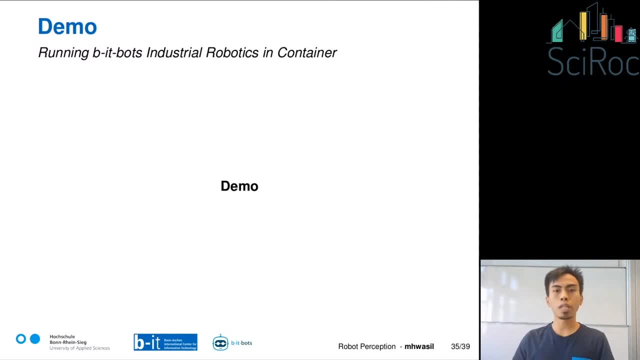 you don't need to install full ROS. You just need rviz and rqt And that's it. You can run our Docker image and then run our perception in the Docker image and then open rviz in your local PC. Yeah, let's start the demo. 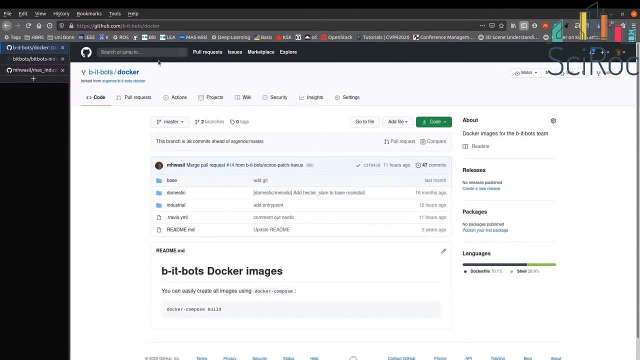 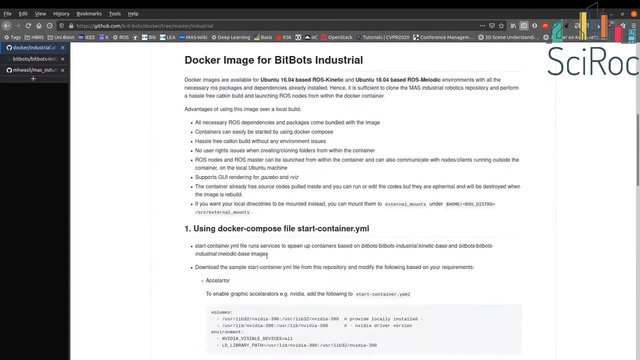 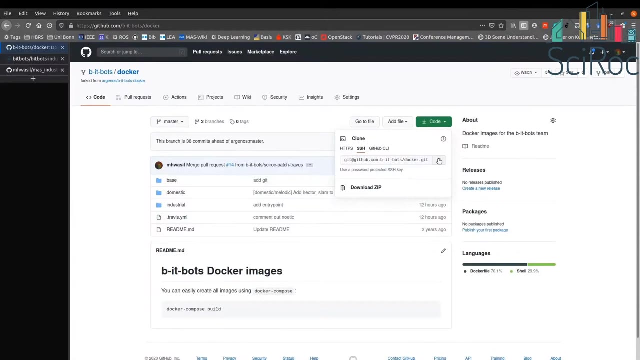 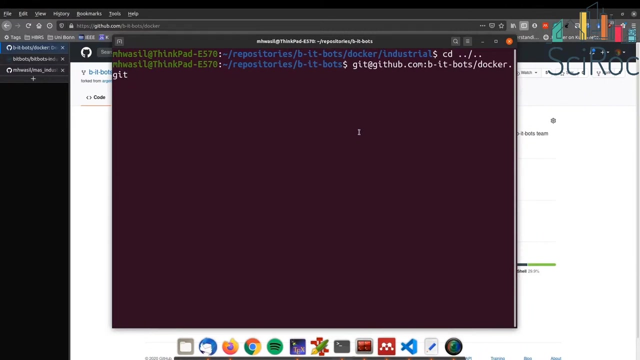 First, let's go to our Docker repository And then clone this repository. We go to the industrial. There is a tutorial on how to use this Docker image And clone this to your local PC, Since I already cloned it, so I don't need to reclone this. 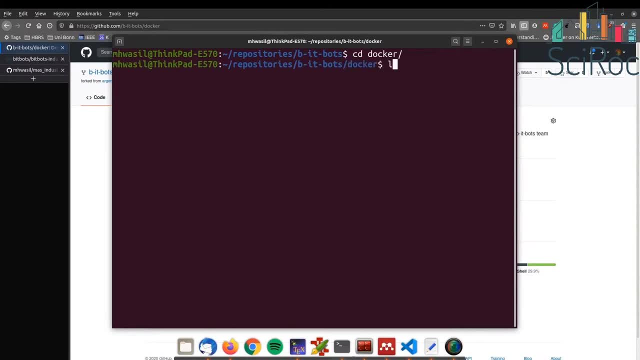 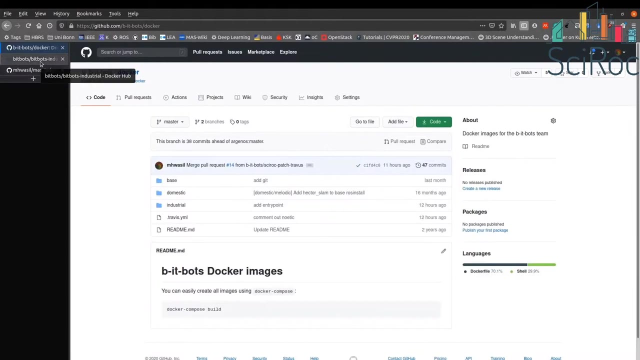 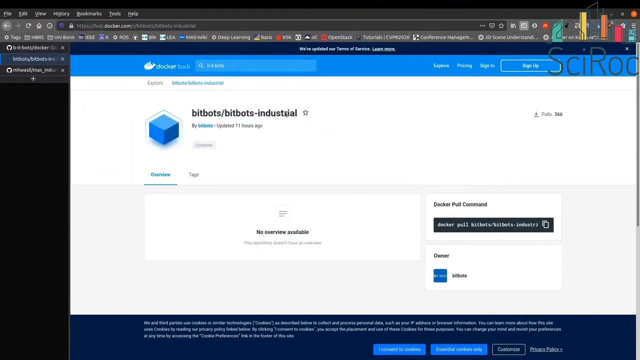 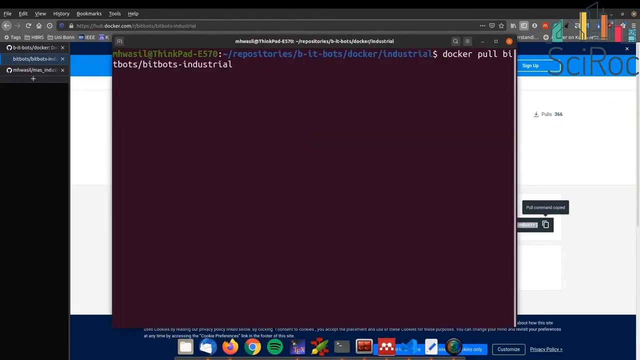 Then if you go to industrial, you should have these files And then next we need to pull our BitBots industrial image from the Docker hub. This is under BitBots industrial. The tag is kinetic base And this will pull the kinetic environment. 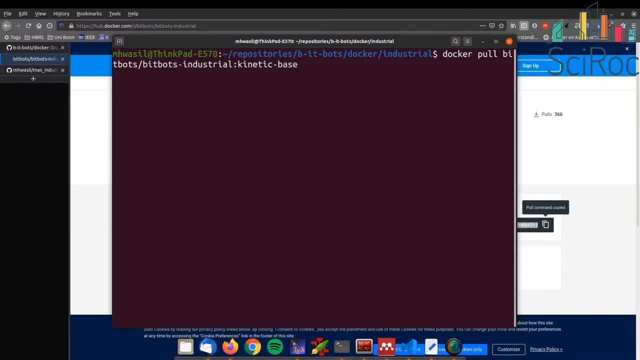 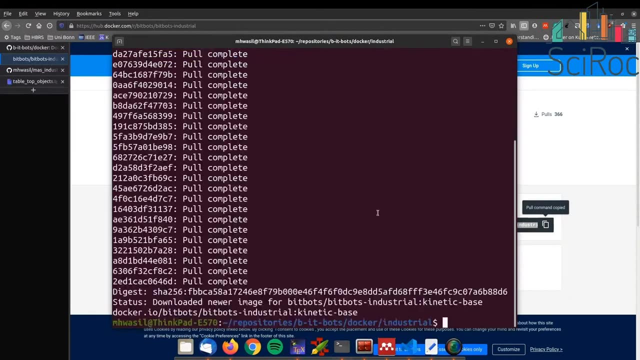 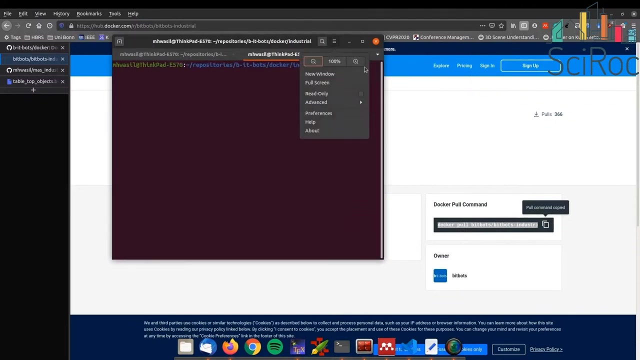 from the Docker hub. So this will take some time. Let's just skip it. Once we get the image pulled from the Docker hub, then we need to pull our unmerged perception packages which we want to run locally in our PC. So if you go to my repository, 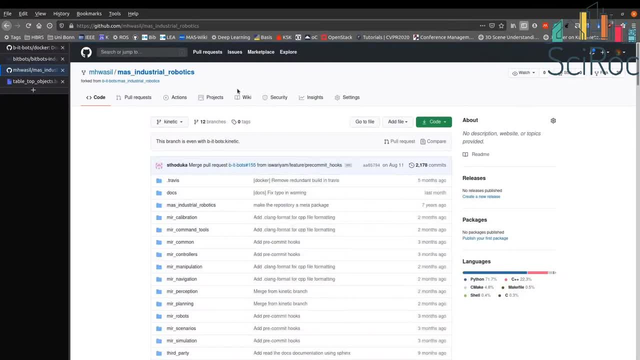 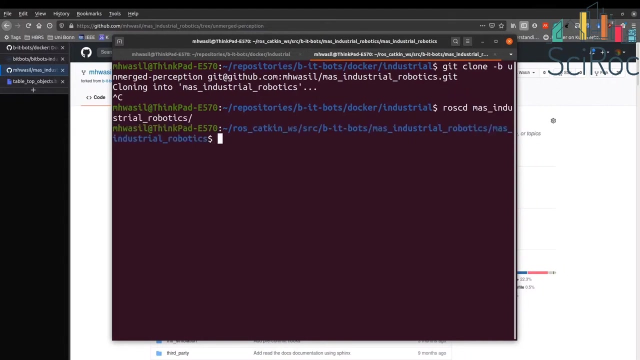 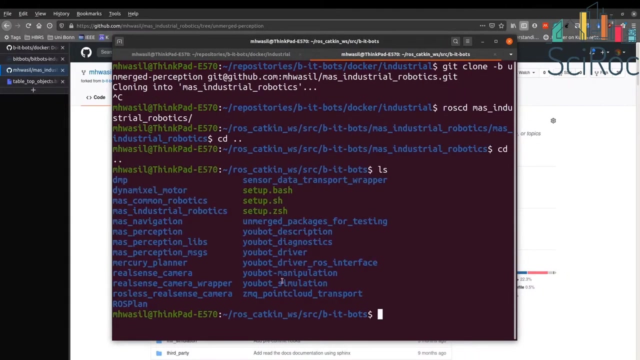 mh1-silmas-industrial-robotics change the branch to unmerged perception And then clone this and specify the branch, Since I already cloned in this PC, so I already have mass industrial robotics. But first let's check the branch. 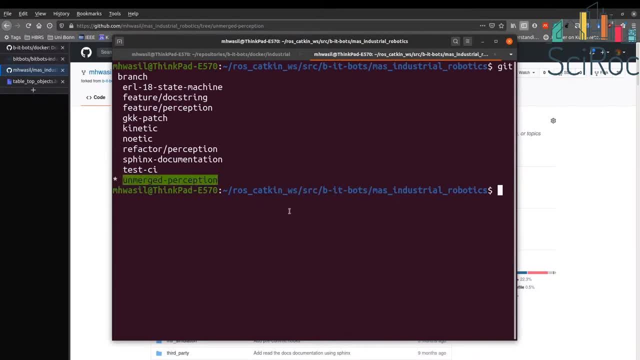 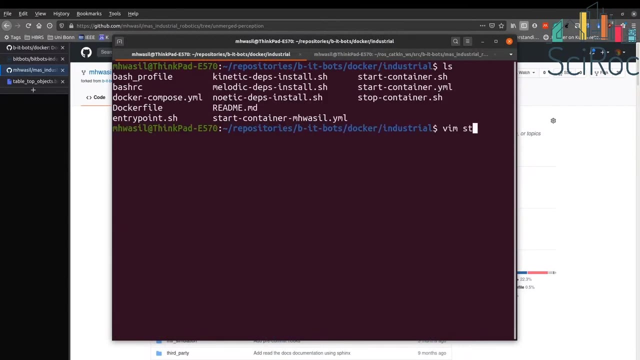 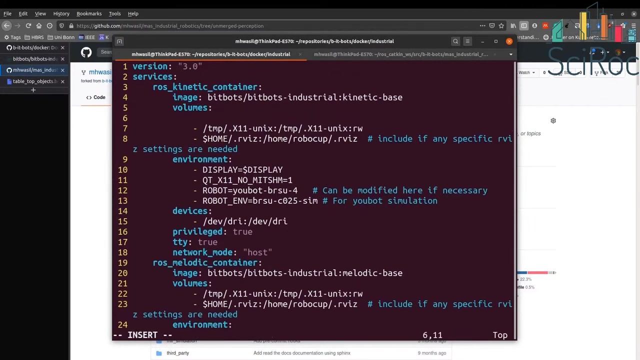 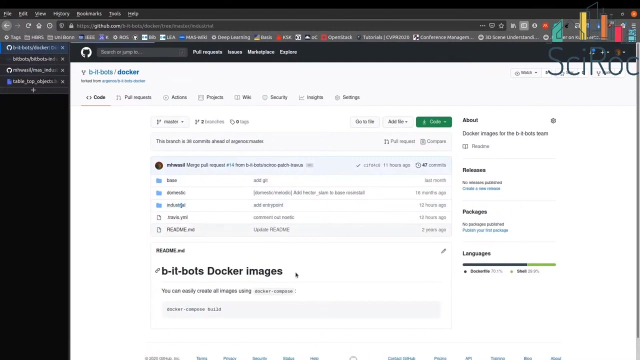 Yeah, we are in the unmerged perception- Then copy the path of this And then go back to the Docker hub And then in the startcontaineryml and then under volumes- ROS, Kinetic Container- Add that volume. So there is an instruction here. 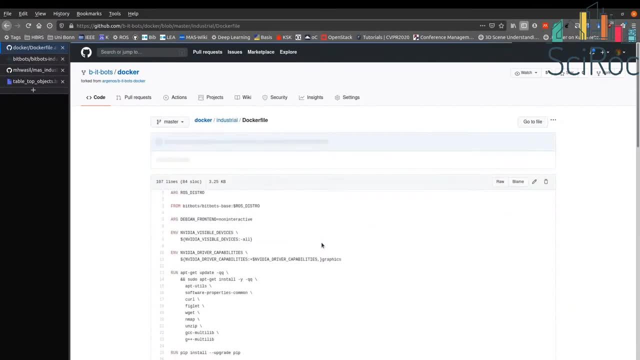 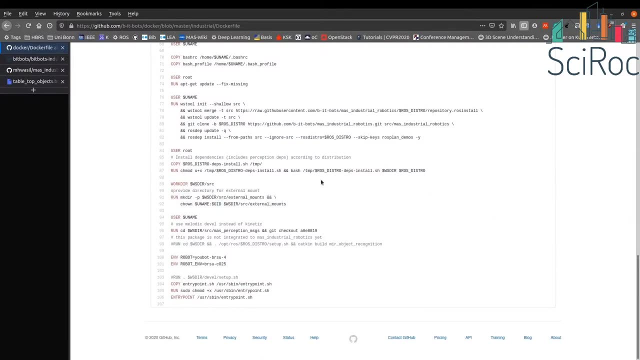 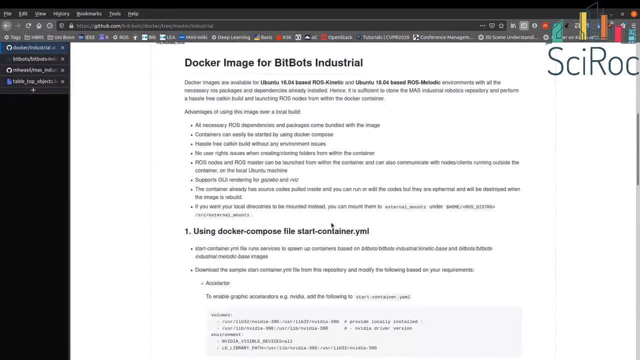 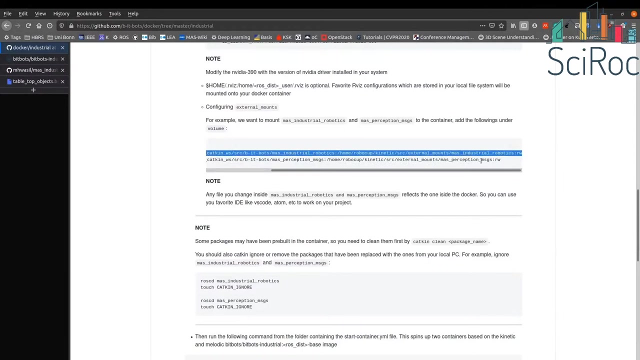 on how to mount your local packages to the container. So we provided an external mounts in here And this is on by RoboCAP so that you can read and write, And these changes will reflect your local changes as well. Let's just copy-paste this and then. 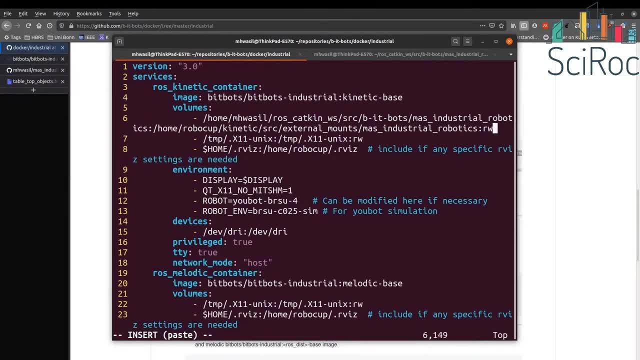 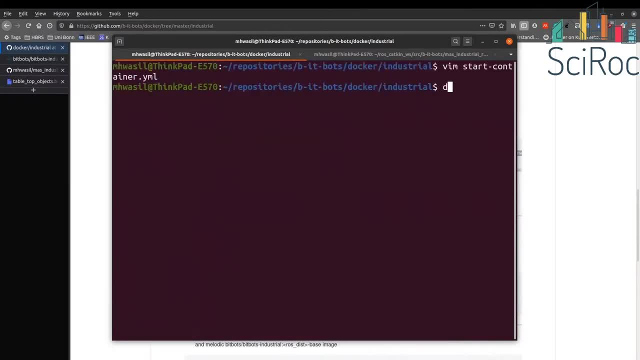 and this will be mounted to RoboCAP Kinetic External Mounts. and the permission is read and write, And that's it. Let's bring the container up, first By docker-compose, and then the file startcontaineryml up and then the name of the container. 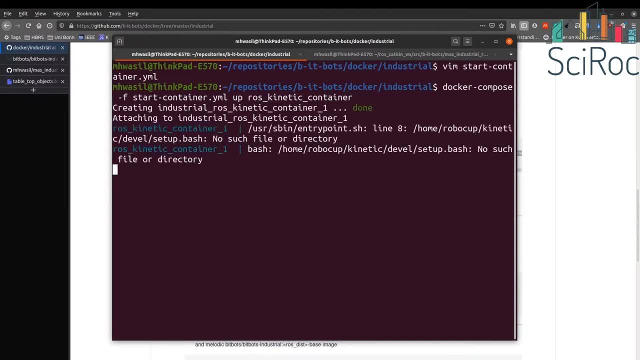 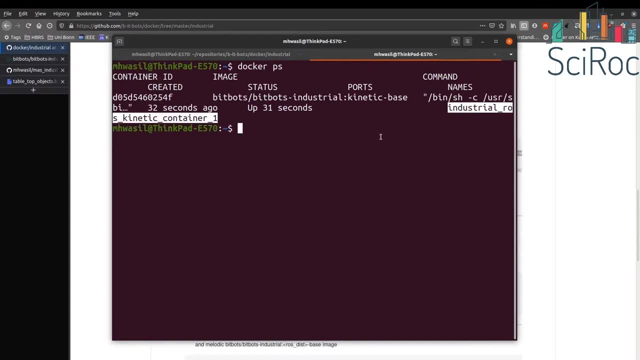 ROS Kinetic Container. Now check if the container is running. So just copy-paste the name of the container, Then just log in to the container by docker-x and then the name of the container. So now we are in the container, So we will have. 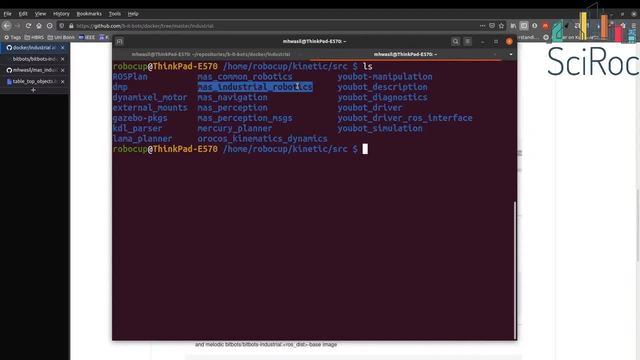 Mass Industrial Robotics. Just remove or catkin, ignore this one, because we already have this in the external mounts. This is our local package In here. let's just remove this Mass Industrial Robotics. Once it is removed, let's just build this catkin build. 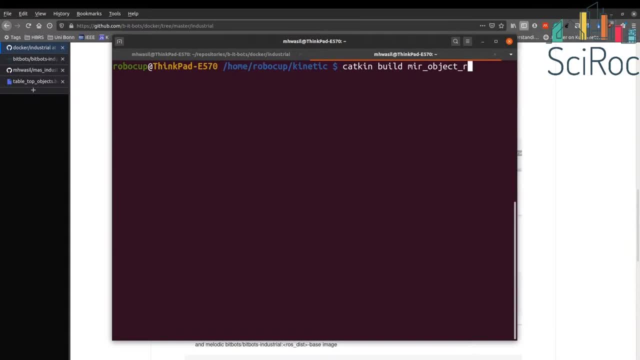 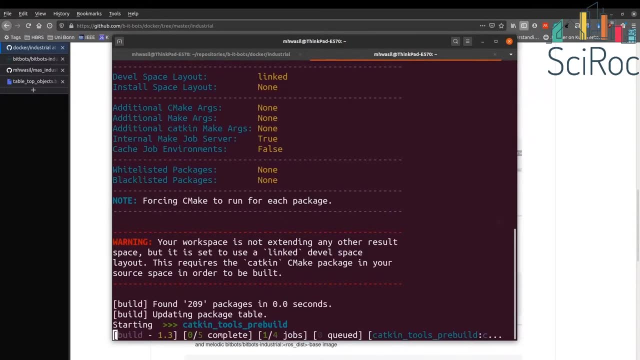 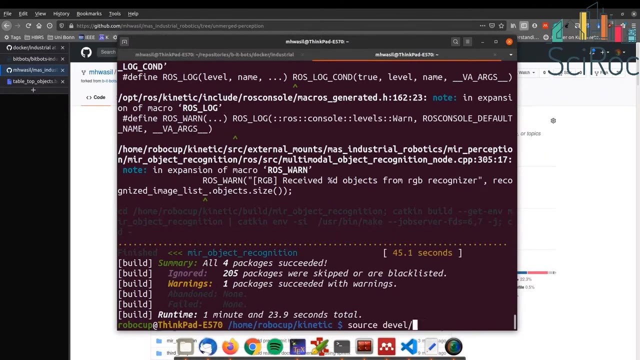 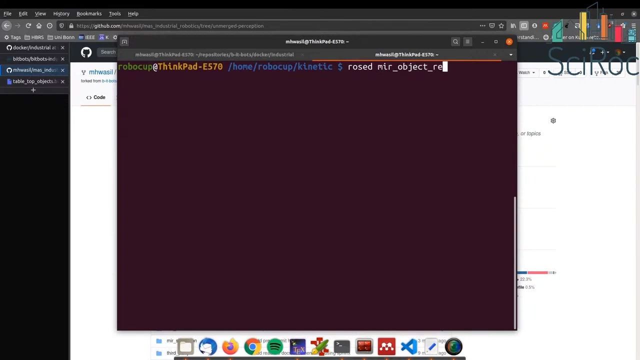 main-object-recognition. The name of the package is main-object-recognition, And this will take some time. Once it is done- source-devel-setupdash- Then we can check what object-recognition model we used. First we can change the RGB. 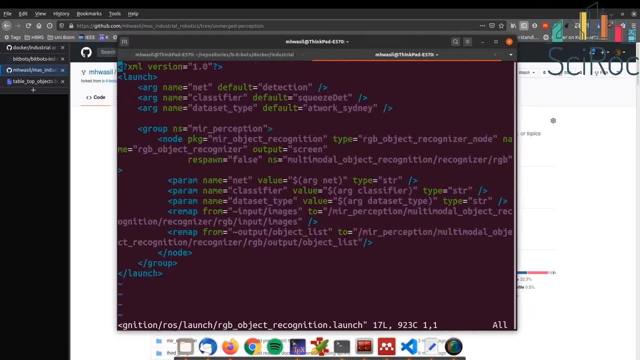 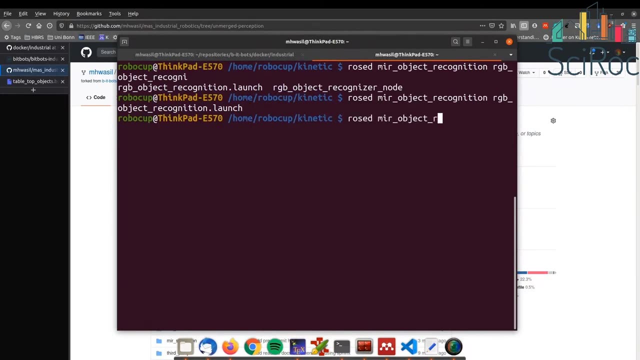 So in the RGB we use a Squished-Date classifier and the dataset is at work-sydney. And then for the 3D rosette-main-object-recognition, point-cloud-object-recognition-node, And then here we have, the model is CNN-based. 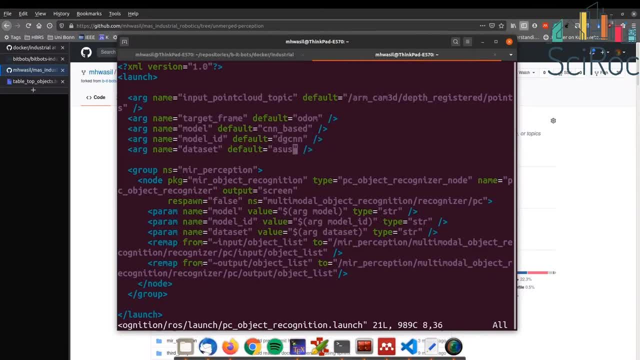 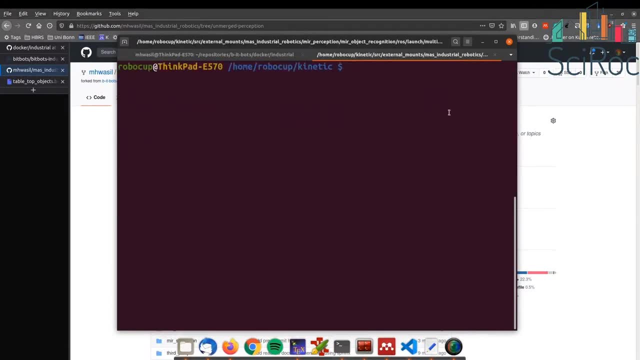 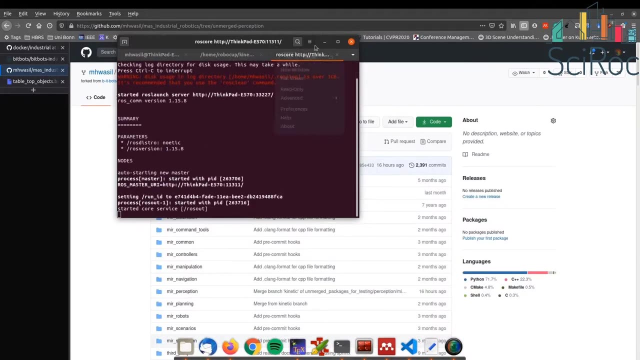 and then the model ID is DigiCNN Dataset it has. Then we need to launch a ROS code in another terminal Just to make sure that it doesn't get killed when we kill the ROS launch. This ROS code is running locally in my PC. 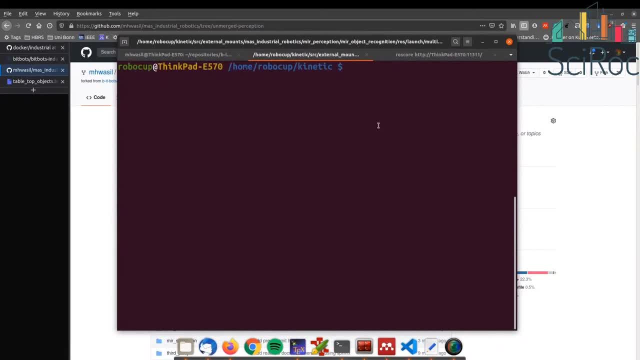 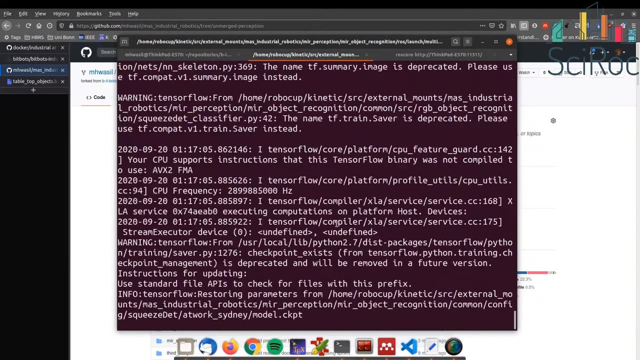 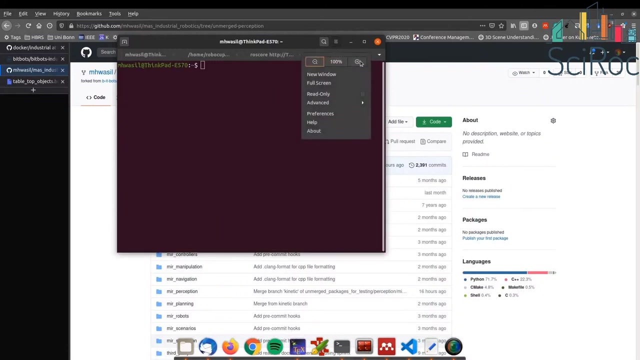 And as you can see here, this is Noetic. Then now we can launch the multi-modal object-recognition node. So this multi-modal object-recognition node is running in the container using Kinetic. First let's launch the back file, Because I already 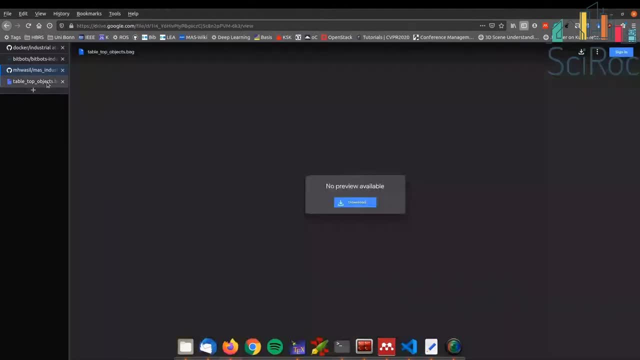 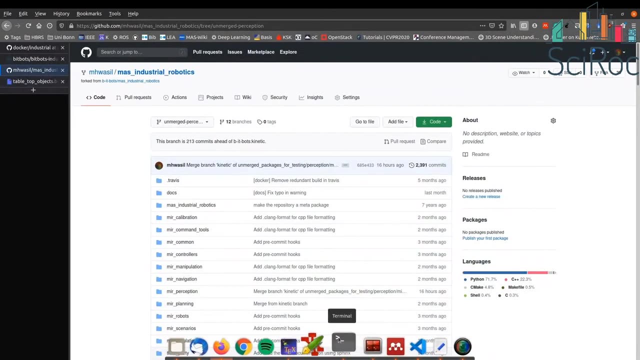 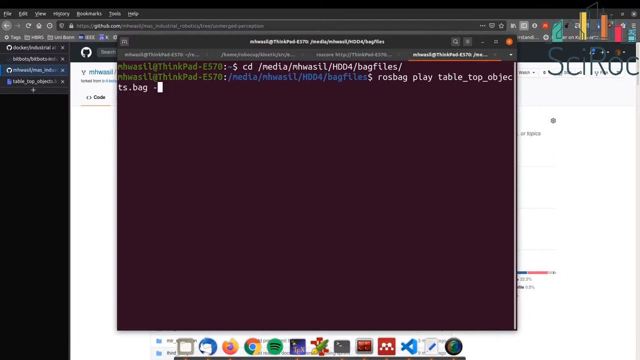 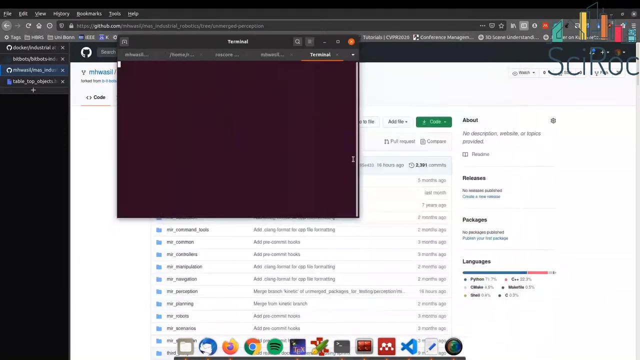 recorded the point-cloud and image data. you can download this from this link. Cross back play and then the name of the back file. So once you get the back file running now you can see that. now you can check Arvis. 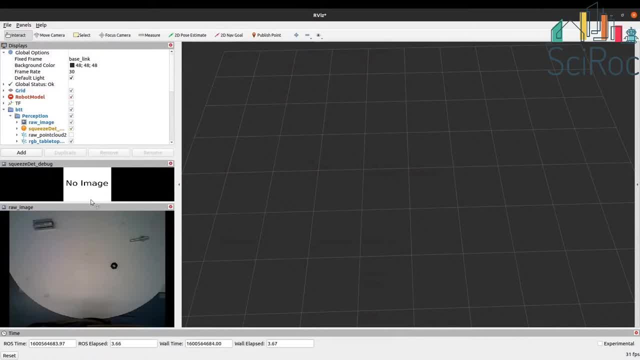 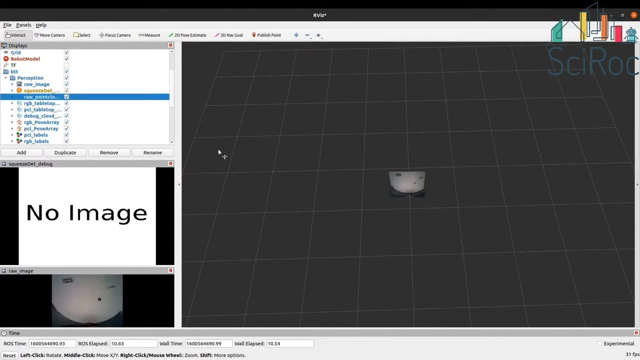 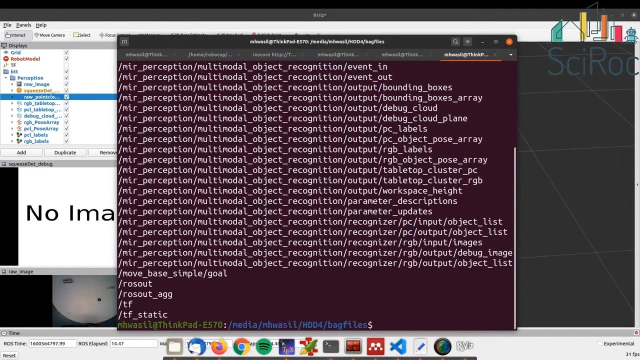 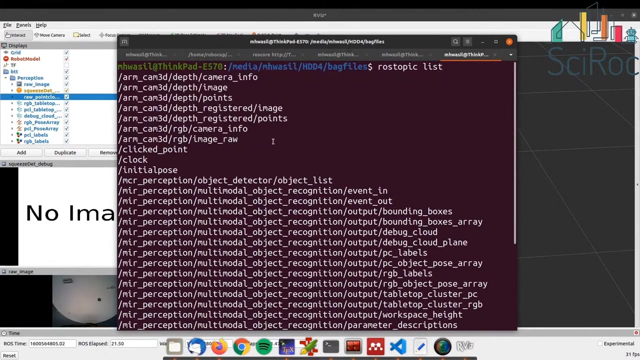 So here, check the raw image, And then we can also check the raw point-cloud. So now check the topic. So now we have this topic And this is the topic from the camera. This is the point-cloud and the image. 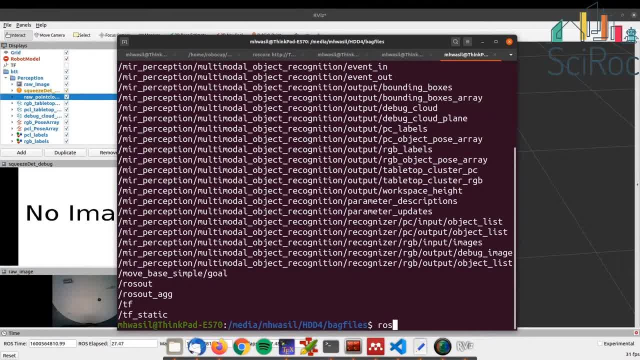 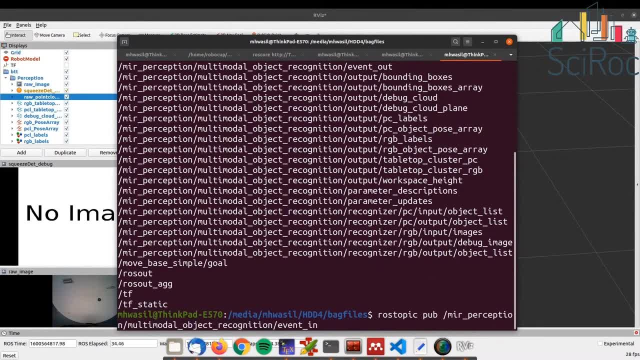 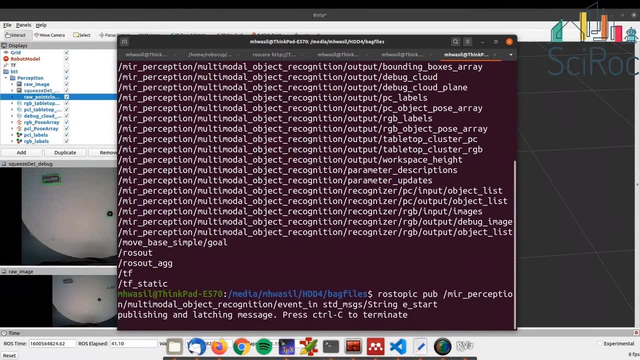 And then we need to trigger the multi-modal object-recognition to Eventain by publishing, by sending e-start to the Eventain. Then it will start recognizing the image and the point-cloud, As you can see here. so we have on the left. 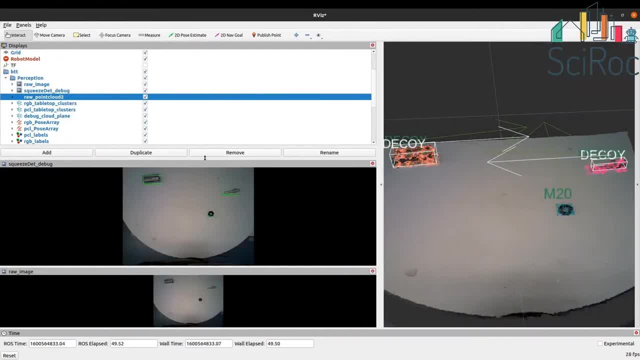 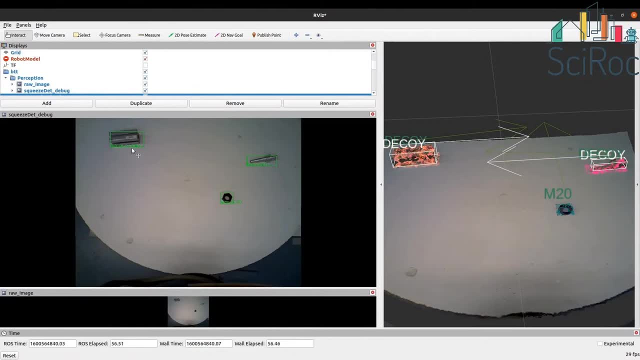 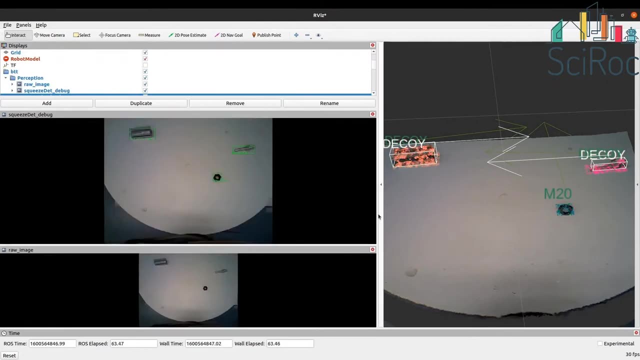 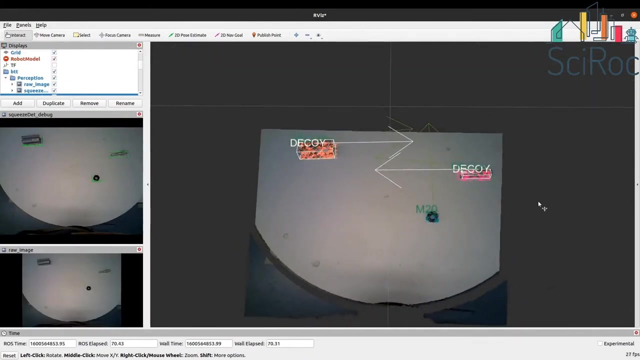 we have the RGB from the squeeze depth. So it detected three objects And so we get a correct classification result in here. And on the right side we have the point-cloud. It says decoys, because they are out of region of interest. 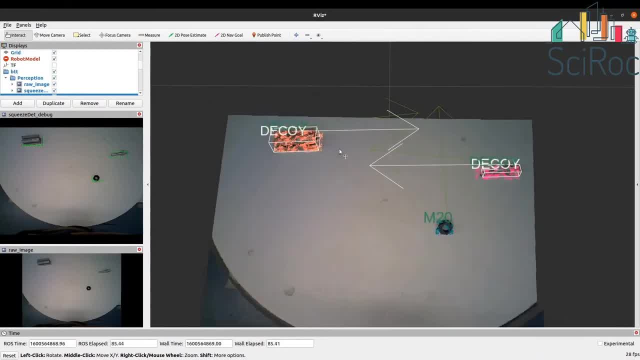 Later I will explain on how to extend the region of interest. The white color are. the white color come from the 3D, while the green one come from 2D. Let's just remove the 3D And yeah, these are. 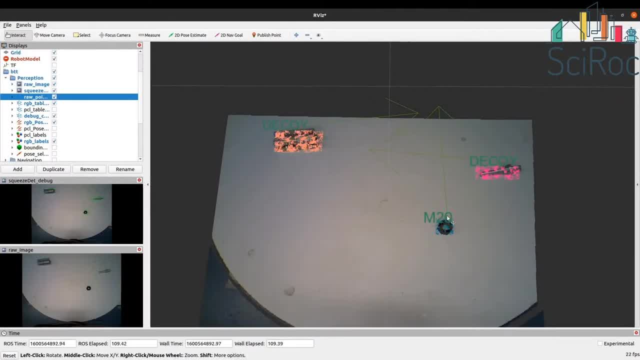 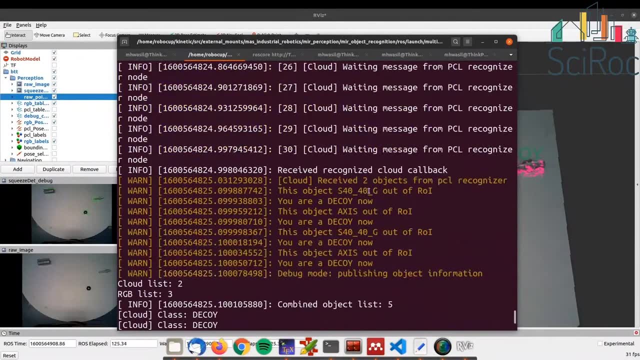 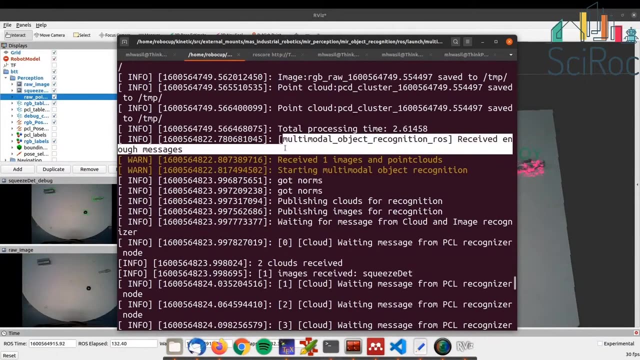 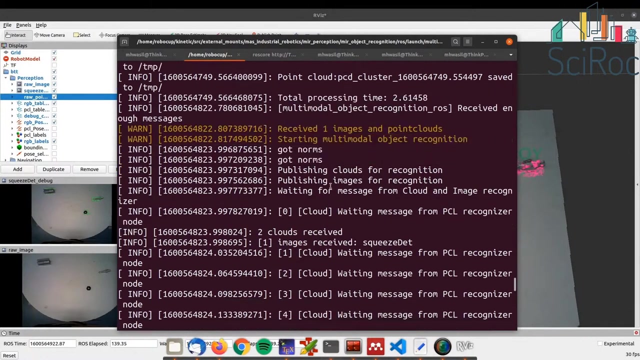 they come from RGB. Let's go back to the terminal. Let's see what's happening. Uh, so what's happening here is that multimodal object recognition get triggers and then subscribe to the point-cloud and image using raw message filter: Start segmentation. 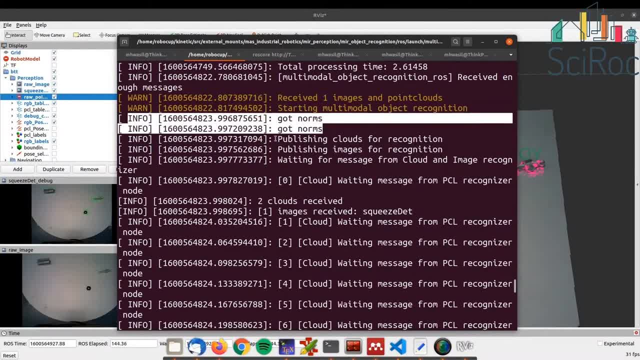 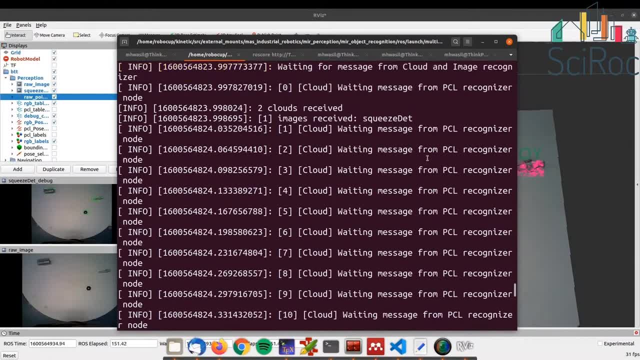 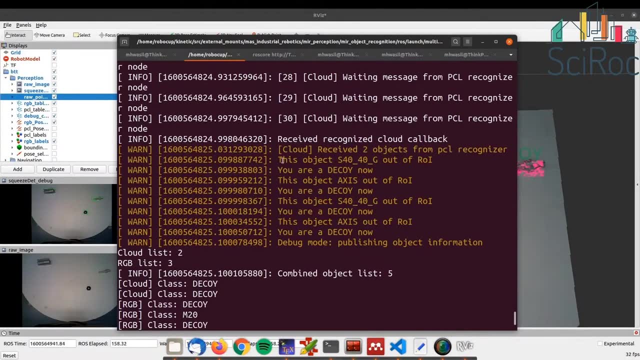 and then publish the cluster to the 3D object recognition and the image, the 2D image to the 2D image recognition, And then wait until it gets recognized. Once both get recognized, then remove the objects that are out of region. 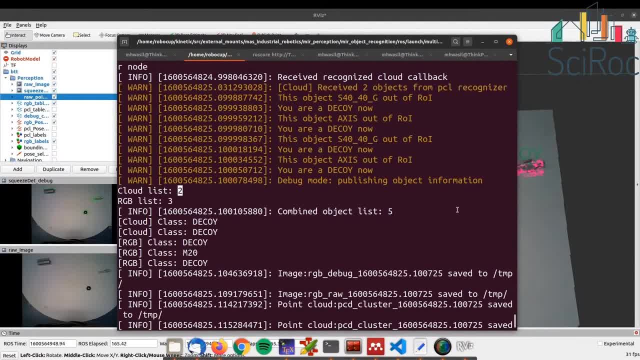 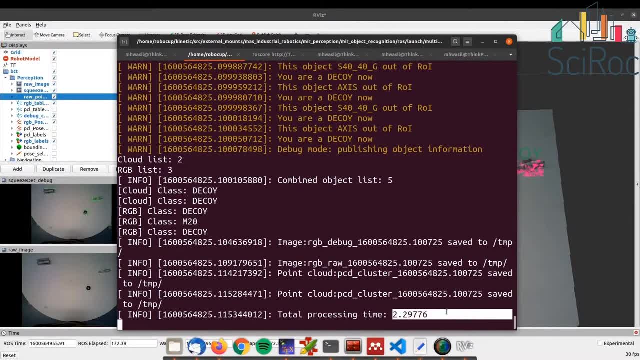 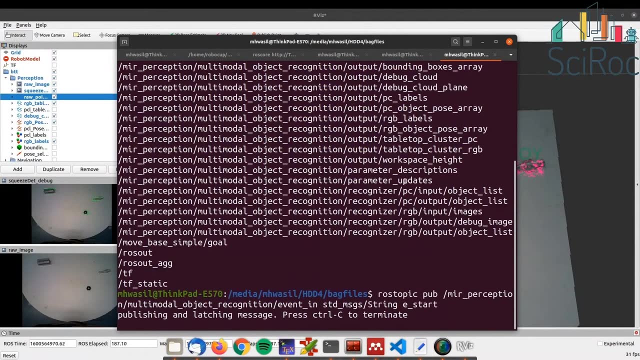 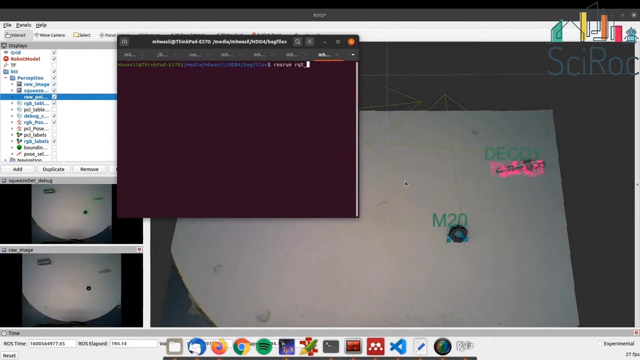 of interest. We have two objects from point-cloud here, because the camera cannot see the small net, and we get three from RGB. So now let's fix the region of interest. So we need to uh update the update, the RQT reconfigure- RQT reconfigure. 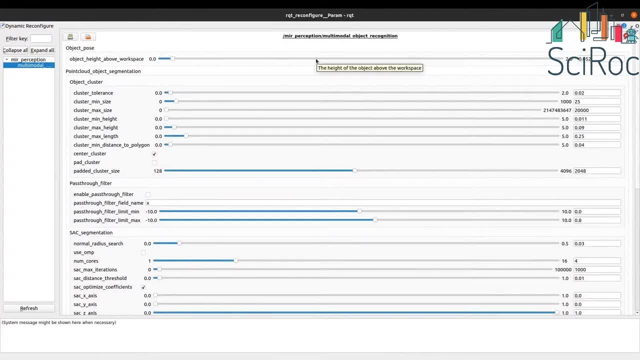 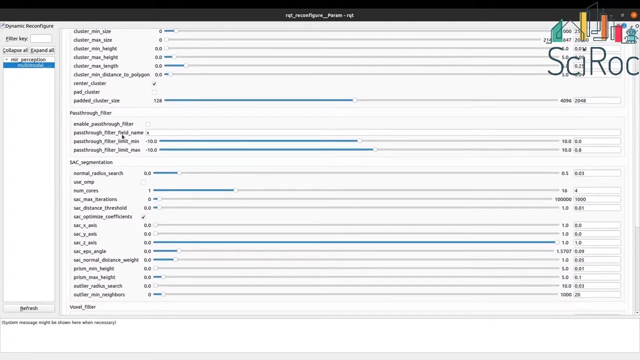 If you run this, you will see a lot of parameters here. So the first one is the parameter to adjust the object height on the plane, And then the second one is the point-cloud segmentation parameters like the cluster, minimum size, cluster and then pass-through. 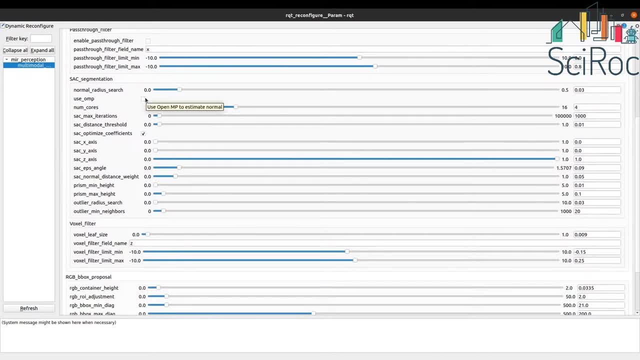 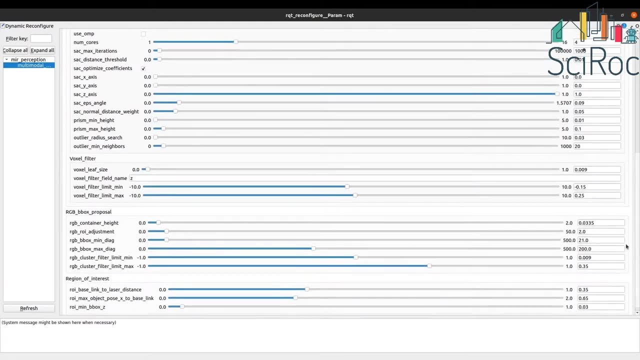 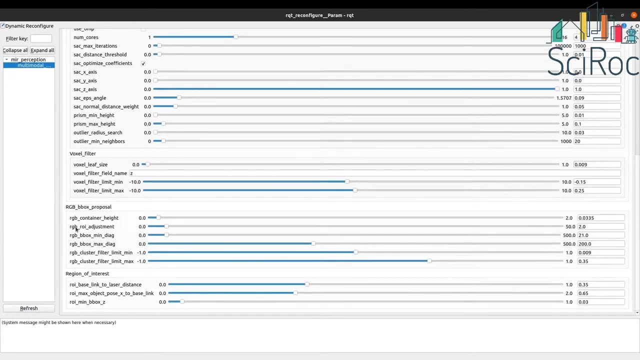 filter, And then this is segmentation parameters, And then we have a voxel filter parameters. here We can also increase the voxel leaf size. Then we have a configuration of RGB proposal. If you want to adjust the bounding box here, you can do this. 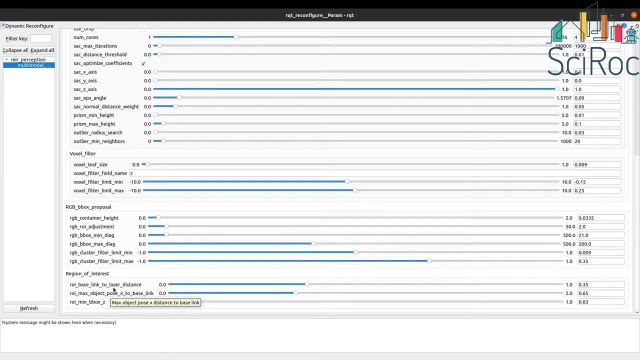 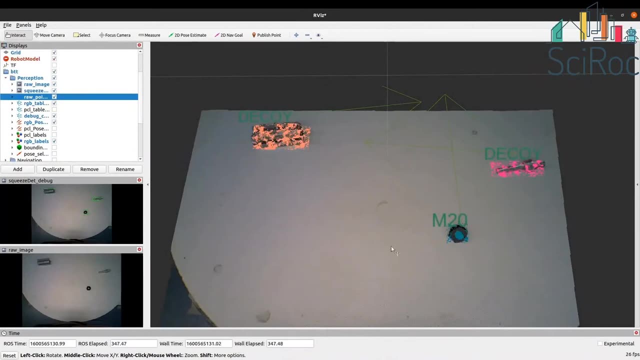 And then, last one, we have a region of interest parameters. So the second one is here. here's the ROI: the maximum object pose X to the baseline, which is the distance of the object to the baseline. If it is out of this, 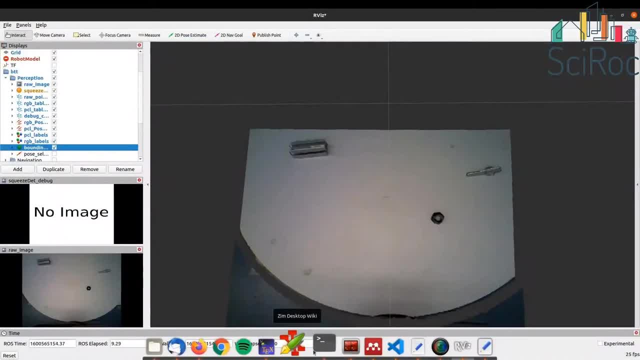 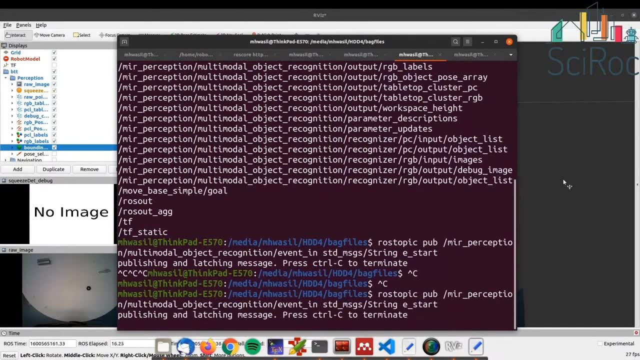 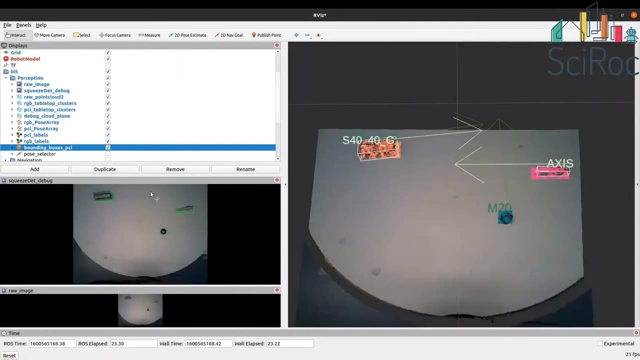 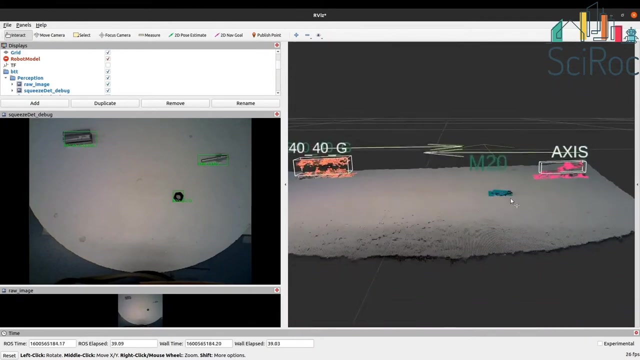 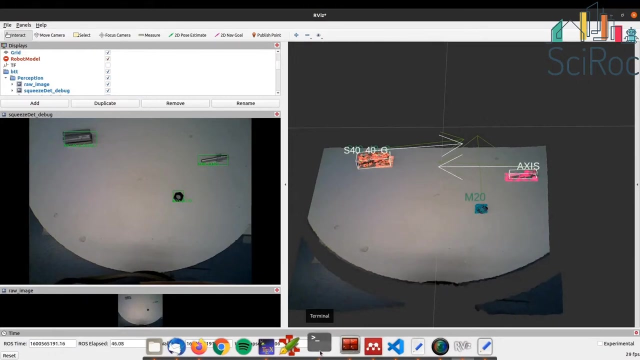 area. this is going to become more dangerous. So we have to find more objects again for the device to create the object or to process it in this place. Before this we have an 3D m20. let's see what happen if we change the, the classifier, let's change the feature based. 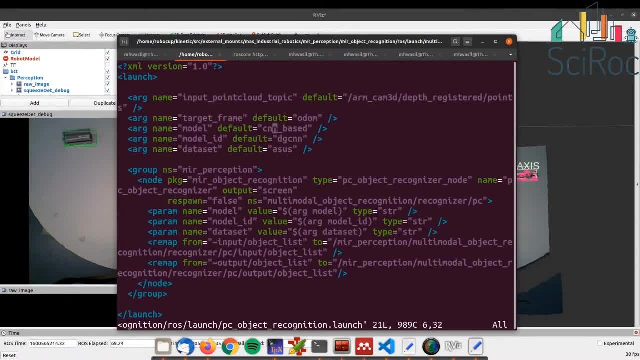 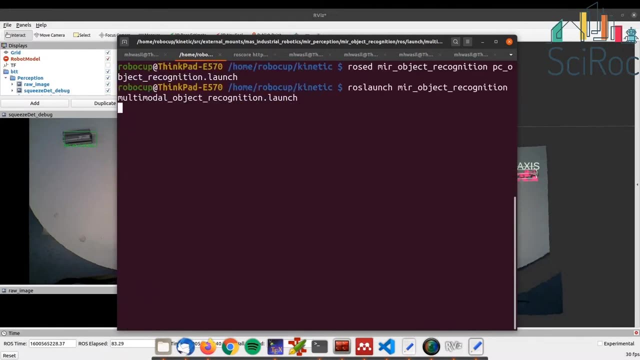 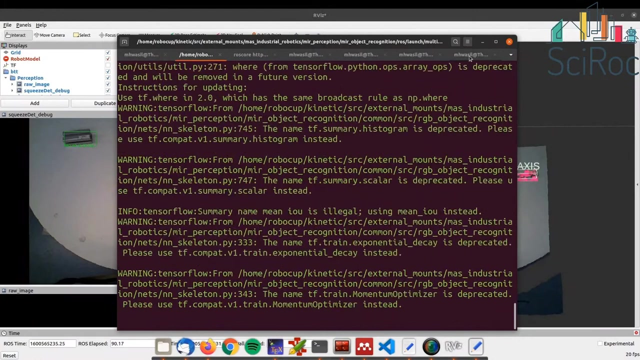 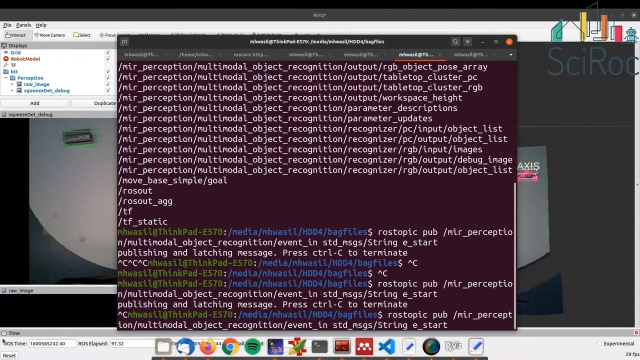 so we want to change the model base to feature based and then the feature, the model id, which is feature factor and radial density distribution, and the data set is axis, and then relaunch the node. so once it is running, let's trigger this again. first let's let's clear ARFIS and then retrigger. 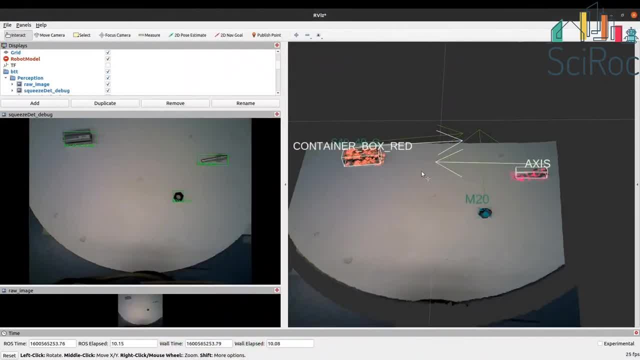 so now the 3d gives container box red here, which means if we do this, everything will be good. now we'll see what happens if we turn on database. now here we'll see what happens if we do this. we'll see if we turn on database. 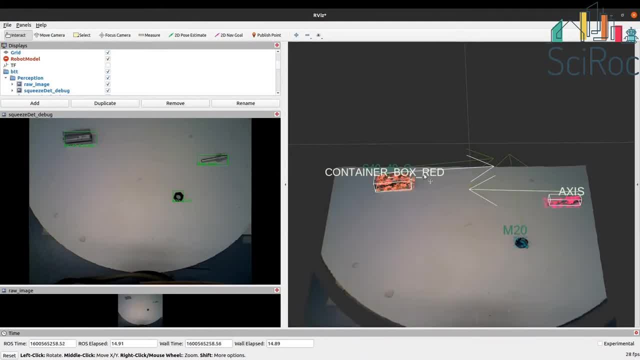 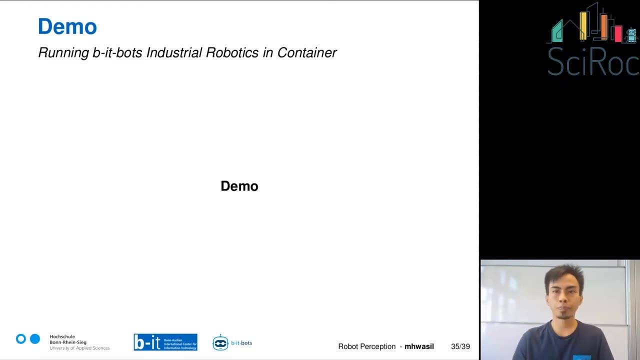 is misclassified. it's actually s4040g is classified as container box, right, but the proposal from the classification from 2d is correct: s4040g. so that's it for the demo. i hope you are enjoying the repo and we. we do have some future works and we because we still have some open problems. 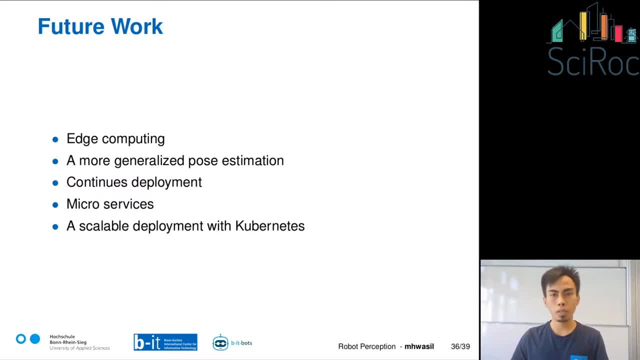 so we want to make the model run on H devices, on TPU or some faster inference, or some H device, some H devices, uh, which can perform faster inference, and we want to improve our post estimation. maybe a more generalized post-estimation is preferable and we want to. 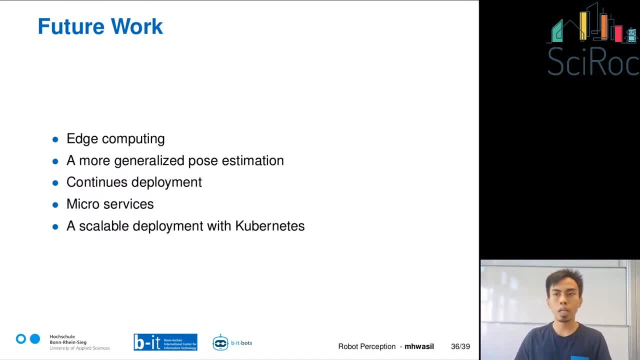 do continuous deployment, such that we don't have have to- uh, we don't have to worry about the continuous integration, delivery and then continuous deployment to the robot. and we want to make these uh components in the robot perception more modular. and we want to move, run this in micro services and use something like kubernetes or 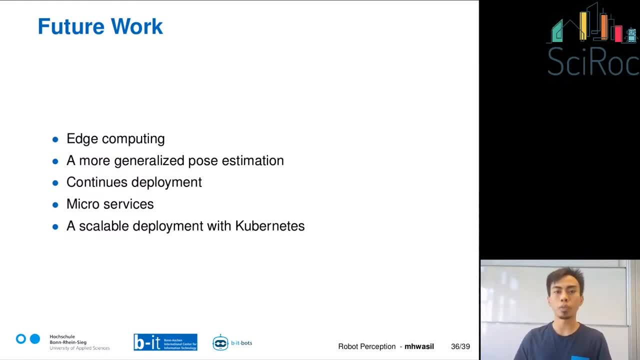 docker swarm to manage them, such that we we don't have this single point failure, because currently it is running on its own. so if the node fails, then we've we. there is no one who will take care of this, so somebody has to come and then rerun the node. that's it from the from the robot perception. 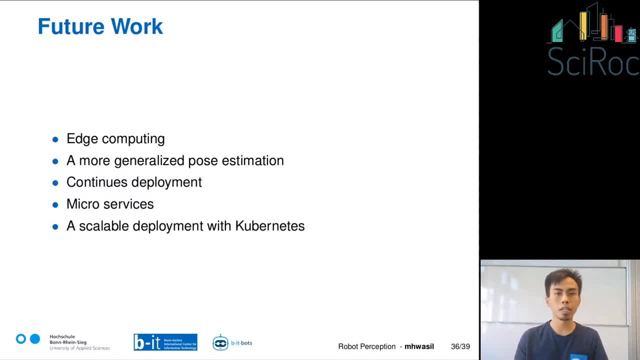 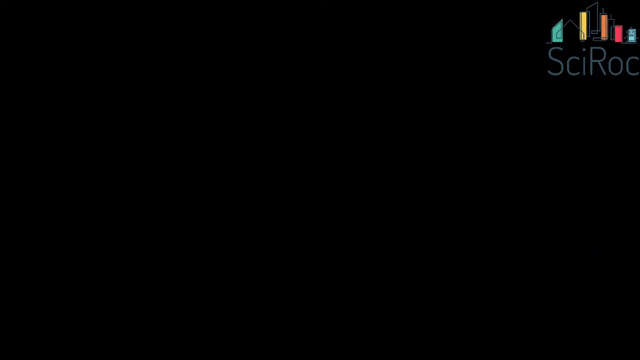 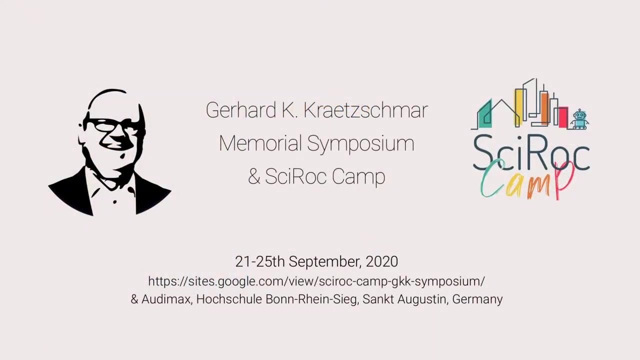 multimodal object recognition using point clouds and images, and thank you for your attention. if you have some question, please ask in the comments or you can also write some issue on our github repository, githubcom. bitbots- mass industrial robotics, or you can also read our documentation in the bitbotreadthedocs. and thank you and stay healthy. 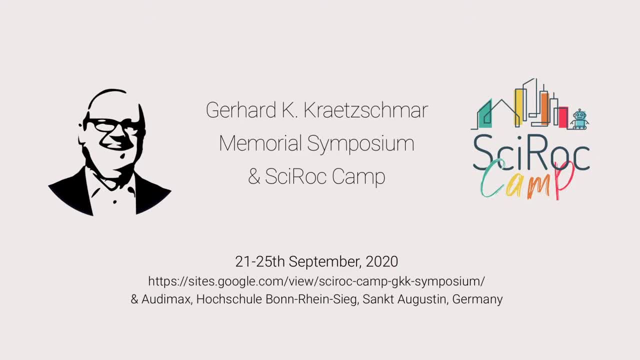 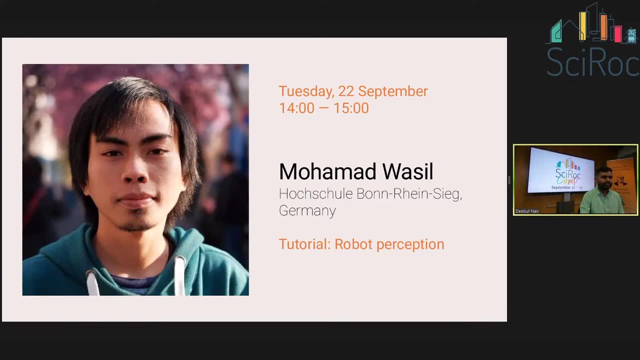 so thank you for the demo, was he, i think? thank you for the tutorial. it was really nice. um uh water. what i really liked was this configuration based setup. so, as i promised to everyone, uh, we have uh, we have been joined live uh by vazil uh, so please welcome vazil. hi hi, how are you? uh, i'm good, thank. 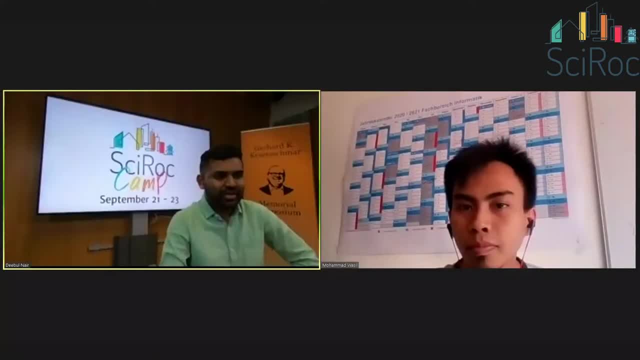 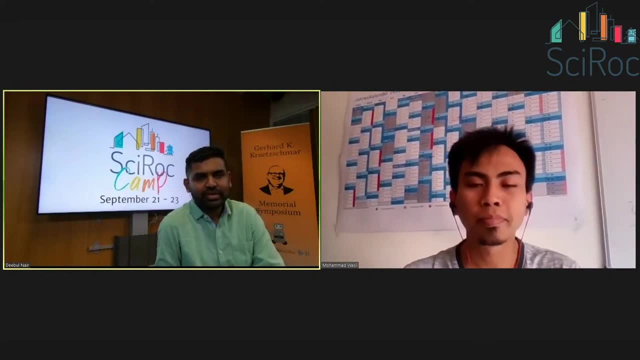 you. how are you people? thank you, i'm also good and uh. welcome to the skyrock camp and first of all, let me thank you for giving this informative tutorial. it was really nice. i think any new team and with even with the demo and the code, i think any new team who wants to. 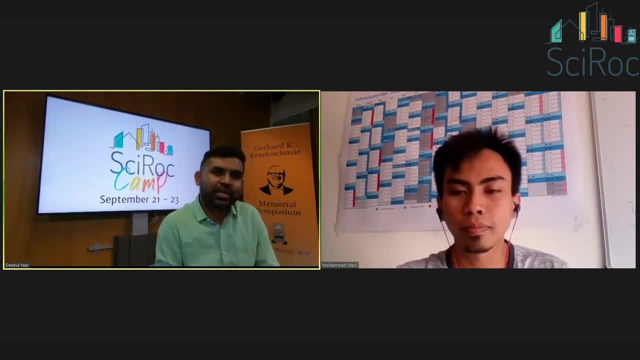 uh, start, i think they can start at the place where you are. uh, so, for the audience, if you want to ask any questions, do use the youtube comments to ask any questions. in the meantime, when the questions are coming, let me ask something which i found it very intriguing. so one thing you said was the the process for data collection. 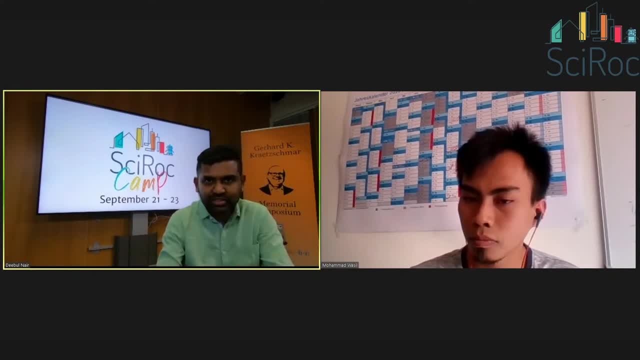 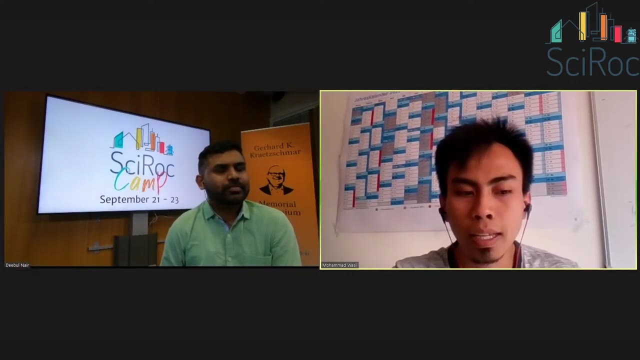 right. so you mentioned it is. uh, so you you suggest us to do feature-based for competitions because it's not data intensive, but still you need data, right? so how is the data collection process for the point? let's say we'll begin with that. yeah, that's interesting question. so we have an automatic data. 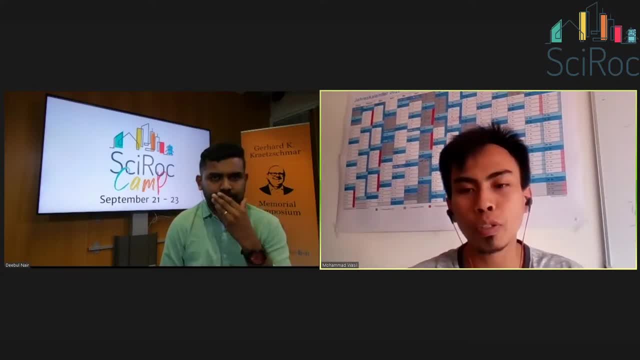 set collections. so we we put the objects on top of a table and then we also use 3d in that case so that we can replace the background later on for augmentation. so that is easy to collect like bunch of data in, you know, in in one hour then we can get. we don't have to label them because 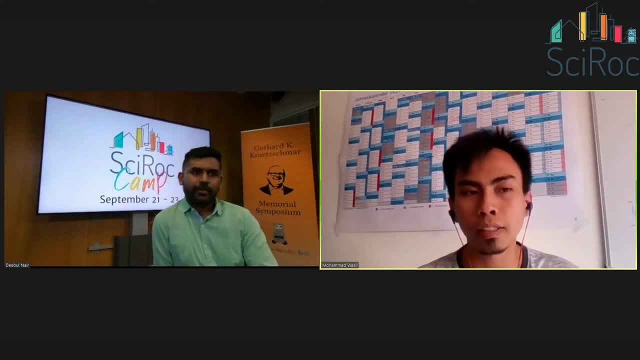 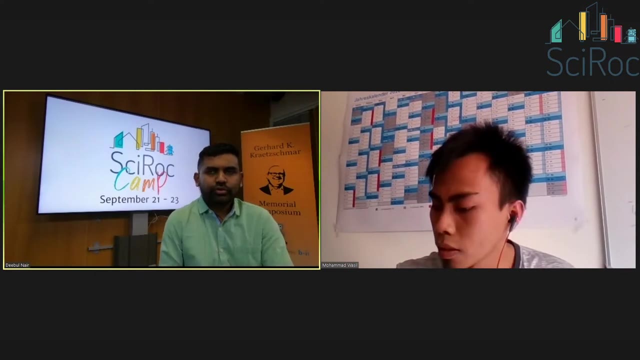 this is automated. this is also open source software and this is done by some students in ms and also some r d students, so this is available also on the, and so do you think the data set you have collected? so does it need to be redone in? 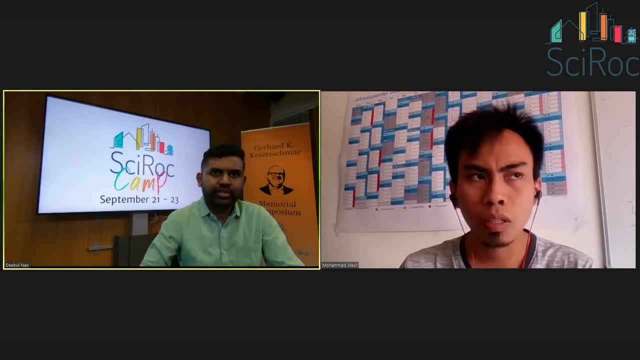 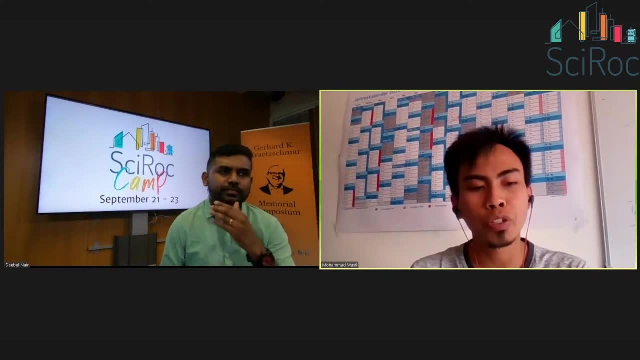 the in the robot place. so do we need to recollect the data set? so it's easy to collect. so, yes, um, in every competition we always collected the data sets, because you know, deep learning somehow fails, does not generalize well in different environment and therefore we kind of fine-tune the model and 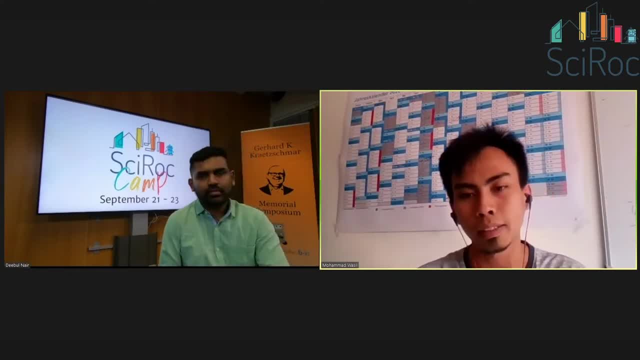 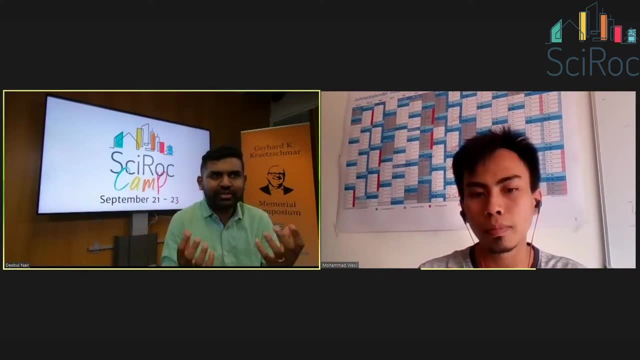 then we collect the data set. that would make the model better, even for the point clouds. you're saying, even for the point clouds, it is the same, because i was under the perception that maybe, maybe, point clouds you don't need. it is the same. yes, but since we use color somehow, like, like, we 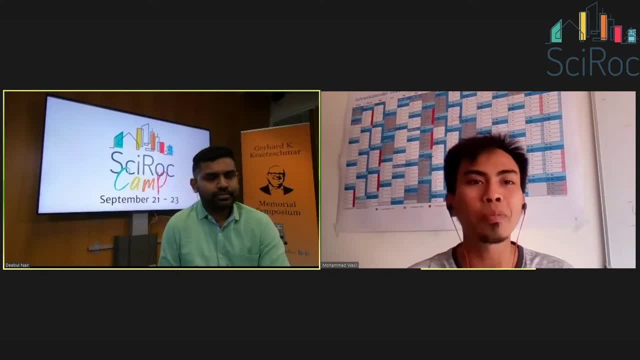 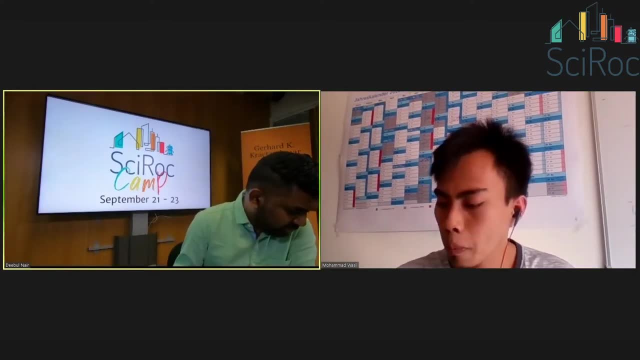 have gray objects. now you have a different lighting condition. it might be it might look white on the camera. so that's one of the problems. nice, so the other question which i was wondering is: so what are the failures, what are the limitation of your feature-based thing? because- and it's very 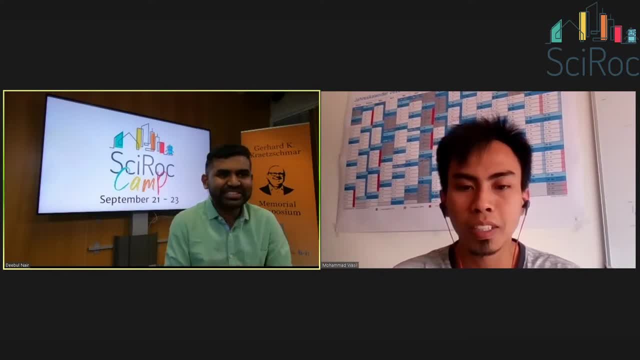 intriguing to know that. you know, in this deep learning process, you know there are teams, who are you still using the non-deep learning? so what are the failures? what do you think? have you faced any limitations? what are the limitations of this? well, um, in general, since we 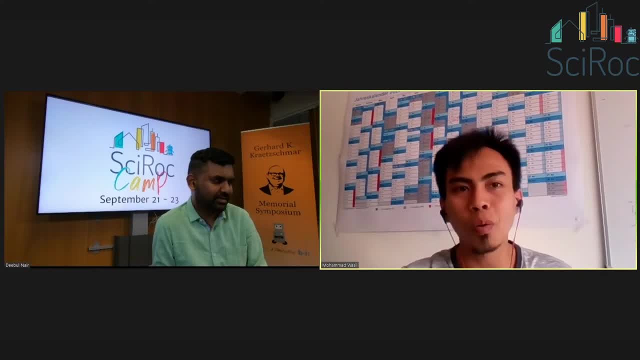 only look once and then pick or whatever, transfer the objects. so it it's not really an active perception where we cannot track the, the position, we cannot re-estimate the pose while the robot is trying to pick. let's say there is a movement on the objects, then we cannot realize that the robot 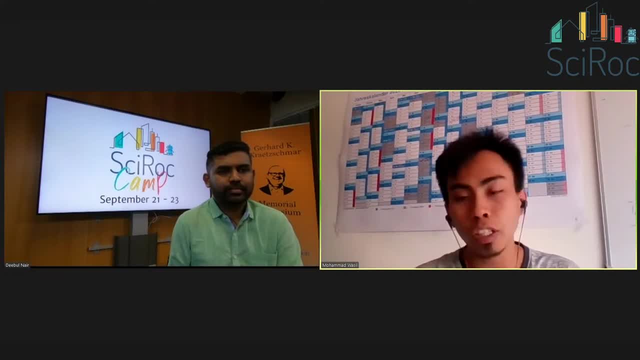 cannot realize that. but if we switch to an active perception, maybe that could help, because we always re-estimate the pose of the object as well as the location of the object, and then we can estimate the position of the sphere between the two objects. so we can double check if we find że, because 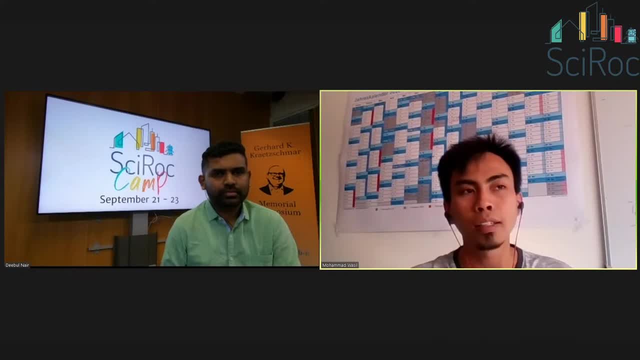 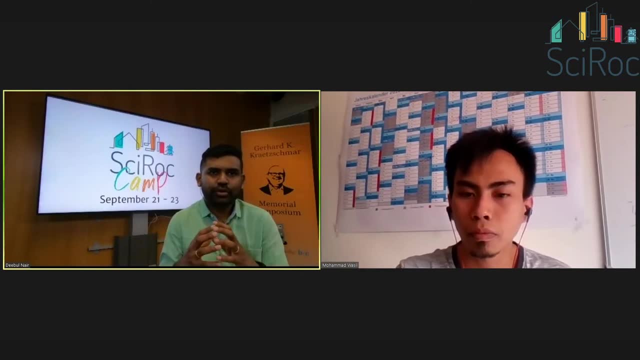 it's relatively blockable. that could also help the model to understand, to get more features of the objects, because the camera is getting closer and the density might be better and the color might also be better. so you, you're saying that you, you are, you wanna, you want to move away from. 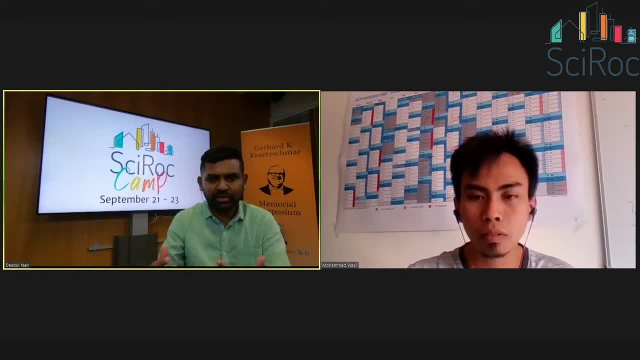 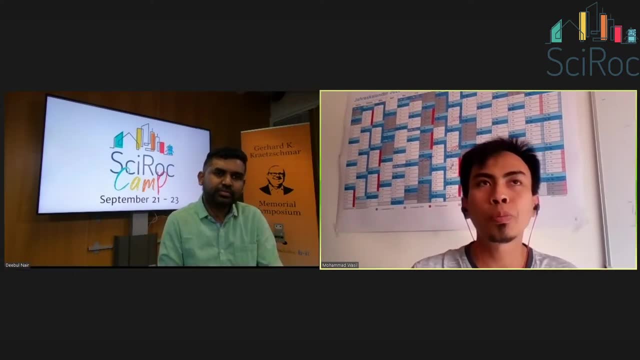 this, uh, this process, because what i understand is that you you perceive, and then you have a pose once, and then that is which is given to the manipulation and you want to processes, yeah, a closed loop. uh, perception and manipulation might be uh better in this case, and 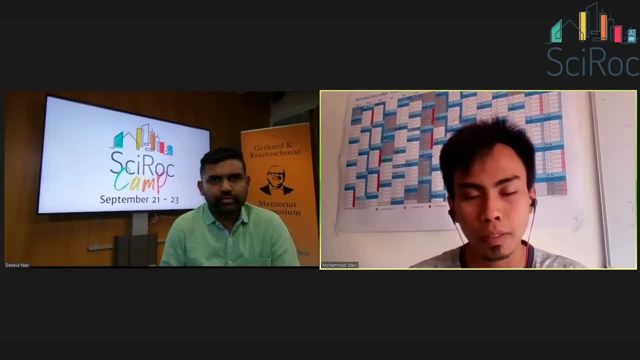 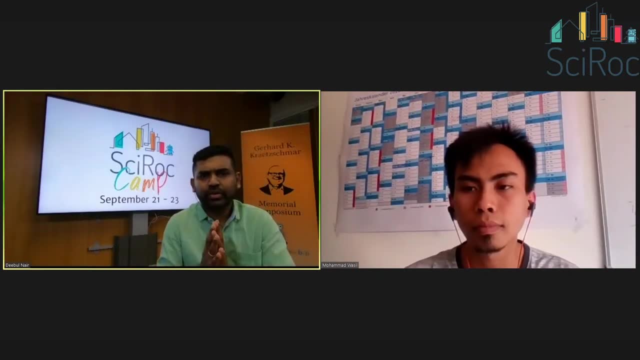 yeah, we, that is our one of our future works right, right. so, uh, in your slides you had a very brief uh thing about um. so, talking about uh, what do you call the uh, since you have this two right, the feature base and then the cnn. so, and then you have talked about how you combine things. so what if 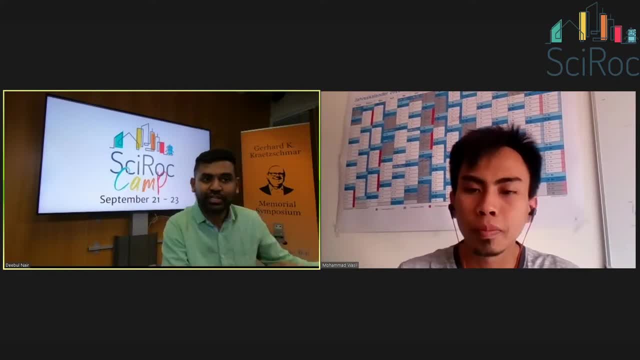 there is a conflict, so so one. so you showed in the demo also that we, we saw, uh, there's a conflict coming from, uh, the point cloud. so who, how do you, who is the the one who makes the decision in that? yeah, and that is, yeah, that is interesting question. so we have an object list: merger. 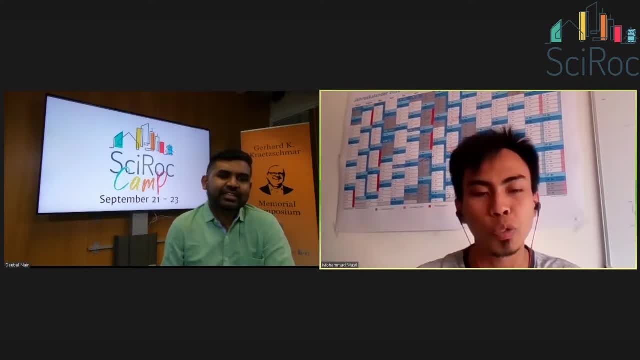 here which merged this uh to result from these two modalities. um, so we have some information, for example, uh, an objects at the location, which we get from the referee box. we get that, that is the facts, that those objects are available on the table, and then we also uh. 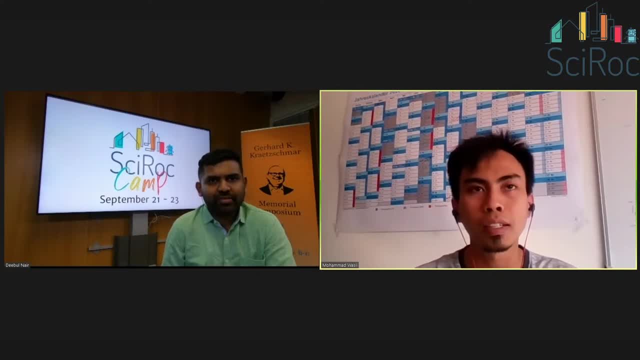 put some something like uh, knowledge, uh, something like uh, we have a rule, a rule base. so, for example, we know that uh point cloud works, uh, it point cloud is worse on recognizing the color of the object, but then we prefer- if they are confused about this- we prefer rgb, uh. on the other hand, if 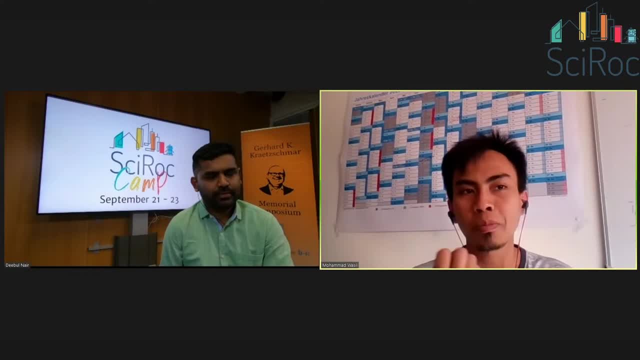 we have a confusion between the shape, for example, small net or big net, then we prefer point cloud, because point cloud works better in that situation. so so you have set of uh rules, uh, with some sort of rule in the object list. yes, so this is like a human rule. we know that. this also, we also have. 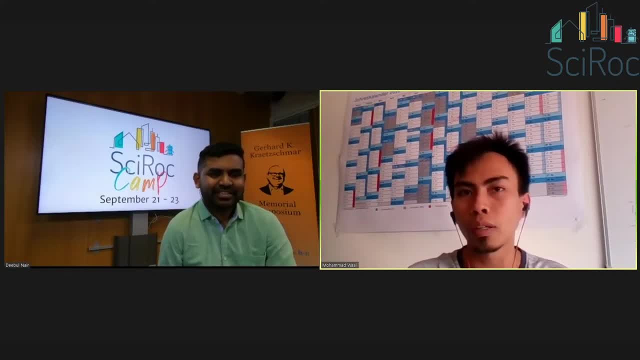 a prior knowledge about the model like model. is this model working better on these data sets or the 3d is better on that data set? so we have that's that kind of information. so what do you think in the future? uh, is that so currently, if i see, if i go around all the robot? 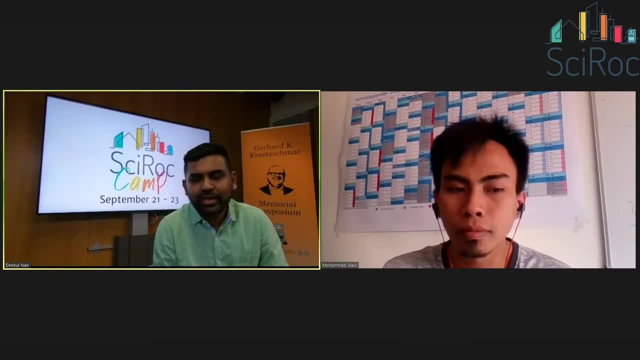 perception has been taken over by deep learning right. so now i come to your team and you're following the point: cloud and processing based methodologies. so what do you think in the future is? uh, do you think there is still hope for doing the basic without deep learning based methods? in? 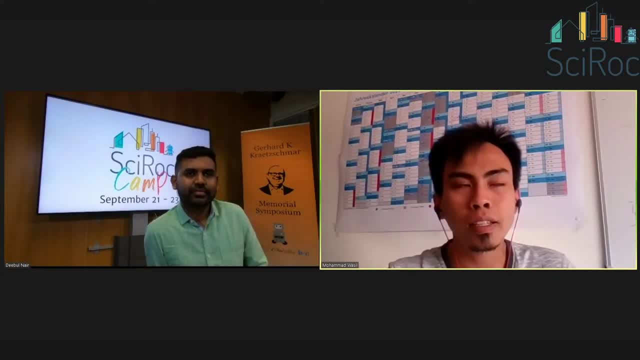 the. yes, of course there is uh at some point, uh, feature-based, uh, classical method is is better, like, for example, in object detection. if we have a new objects and you cannot segment you, your deep learning is totally doesn't work. it doesn't work in the in the situation where the 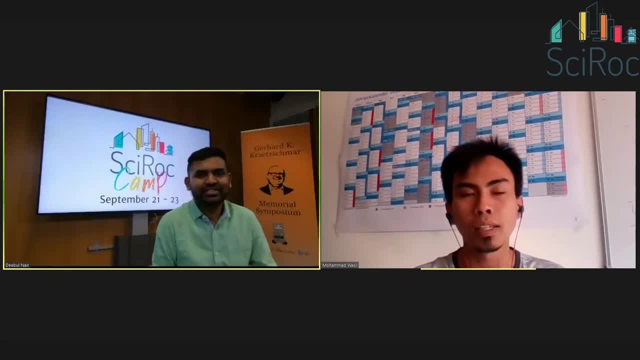 object is. so this is the scalability part of. yeah, the scalability, yeah, and. but if you use feature or some classical method, you can still use it. i think it will perform worse on some situation, but it it will work. yeah, i think the. the right word is not scalability, it is the. it is the time. 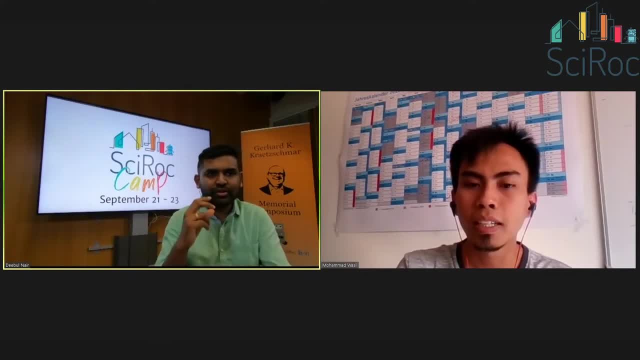 to change. you know the uh to to modify yourself, so it is so the deep learning is, so you cannot change it on your will. you know you have to collect data, so you have to. it's a long process, while on the future processing it is not to mention the time to train. yeah, that's a big problem. 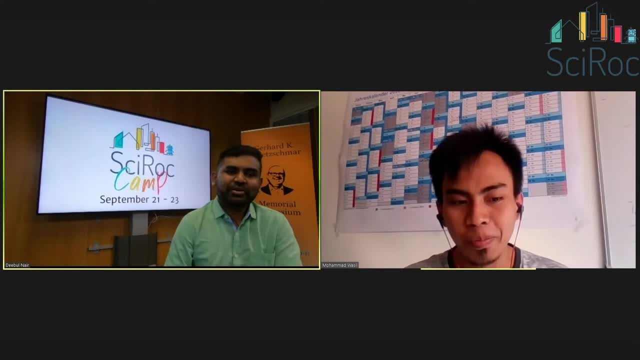 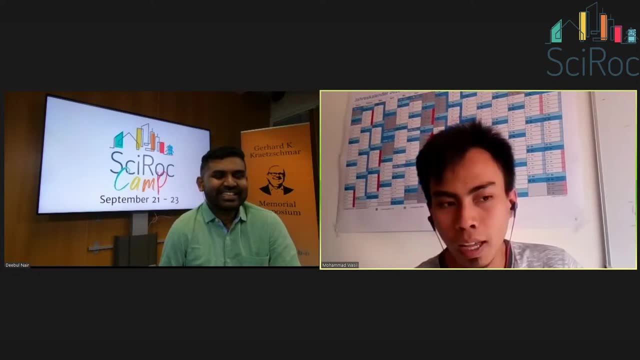 yeah, yeah, like during the competition: what is, what is your time, what, what are your times, how do you train and what? how much time does it take? well, for the, for the squeeze debt or other point clouds like uh, point net or um, and and it takes like. i know it depends on the data set too, but it was mostly like 10 hours. 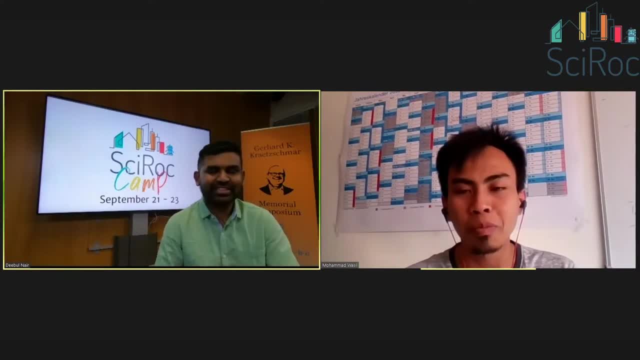 so, but you cannot do this in competition- new objects- then you have to prefer the feature base. that's the solution. okay, nice, yeah, uh, now to talk to consumer: what about the computation power? so you, i know you, uh, we saw the ubot in there, we had the your team presenting and we had shown a bit. 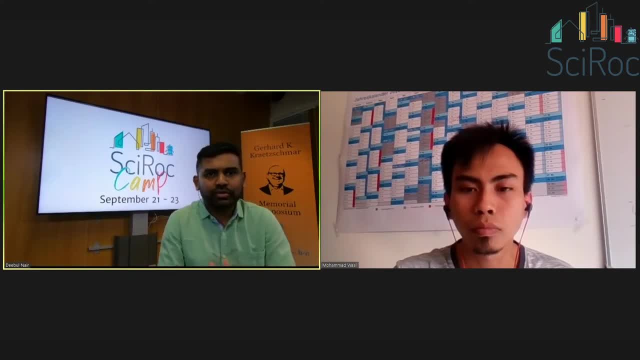 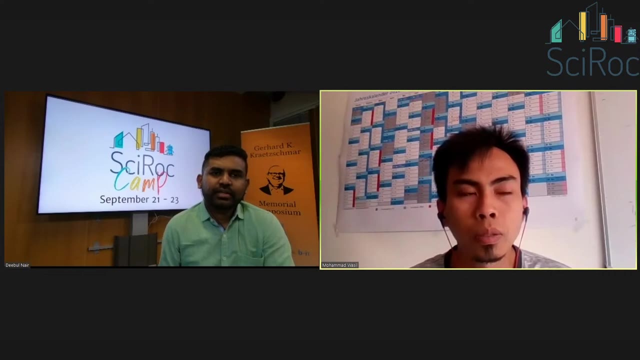 about the hardware we had. uh, it's a nook, which we know from the presentation yesterday. so what, how much processing power is required by, let's say, by the processing by the feature based by the dnns and uh and yeah. so, in, in in total, we it just takes um, uh, it gives us two frames per second, two hertz, the whole perception. 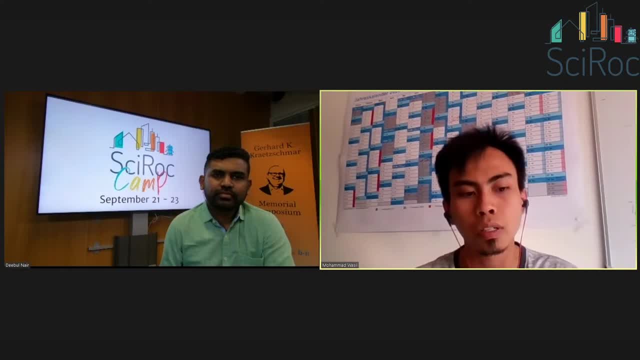 3d, including including the segmentation rgb, the whole perception pipeline. it takes, uh, two frames per second or two hertz, but uh, this can be improved by using a coral stick or a tpu or some other edge computing. so, yeah, we are, uh, we are like working on that. 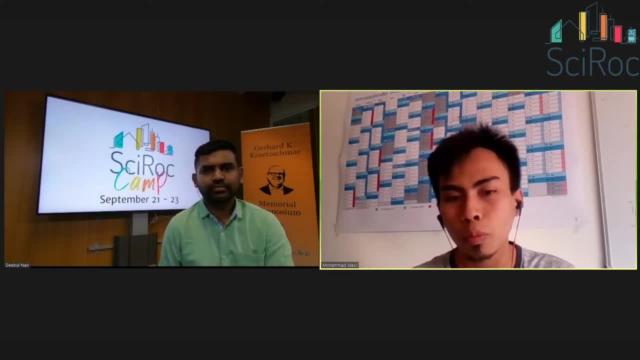 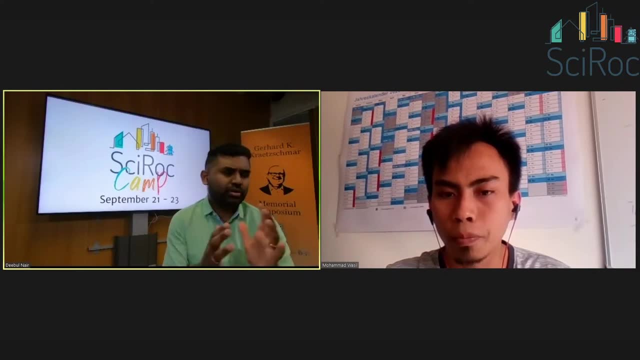 uh to make the point cloud feature for point, cloud models to work on the edge, tpu or edge computing as well. and finally, so i saw you using docker in your demo, which was very nice to set it up. so so is this the standard uh perception, uh way of deploying uh. well, it's not really standard in the 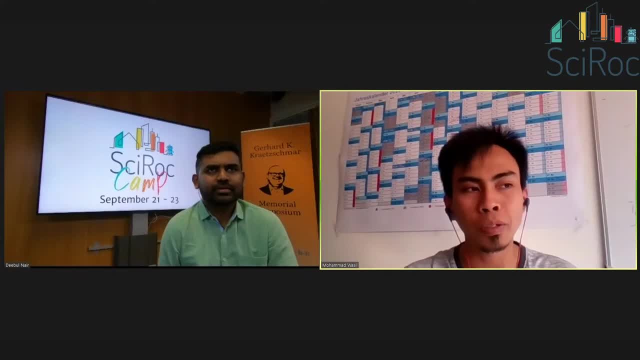 sense because the communication between the house and the docker, it takes a lot of time. you already have raw topic with uh, with the, with the networking as well. so if you communicate between the horse and the docker it might take some time but it might get improved. the the. 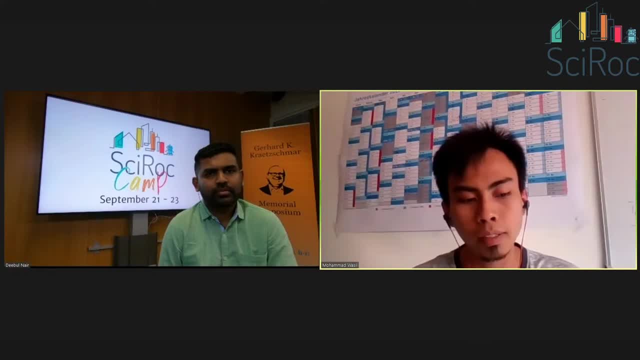 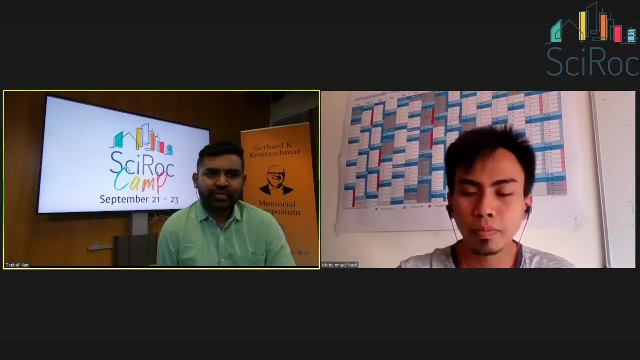 advantages here is that if you we have a docker base, then we don't have to worry about the environment. you can deploy this on any platform because it's just running on its own image, i think. i think we have discussed a lot aspects of it and i wish the whole bigger robotics community 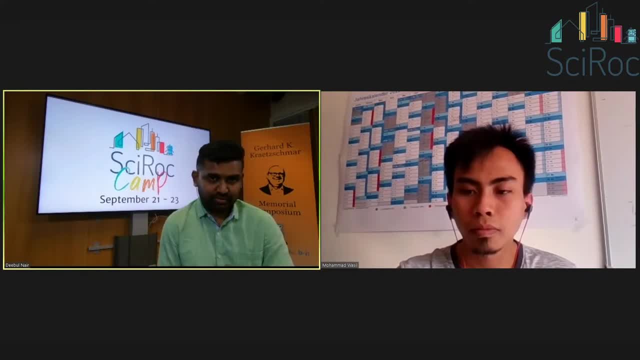 can learn from the experiences and this tutorial of overseas. with this note, i would like to thank again uh zeal joining us today and giving us this uh tutorial, uh, and see you. see you soon in the next competition. so, as you know, we are uh having the next skyrocket competition in bologna, italy, and then we hope to. 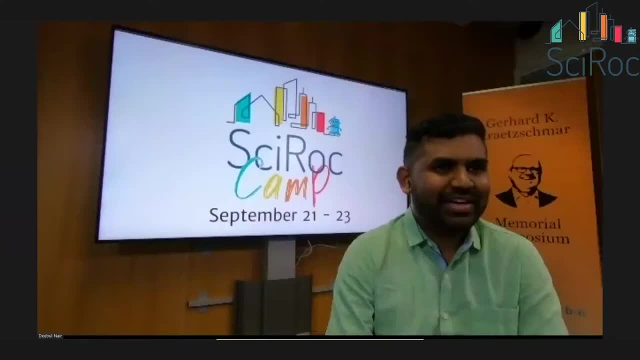 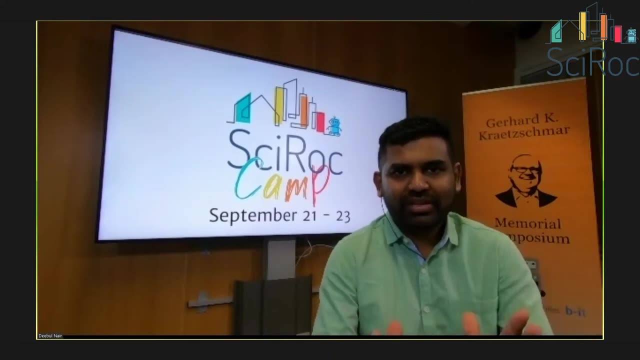 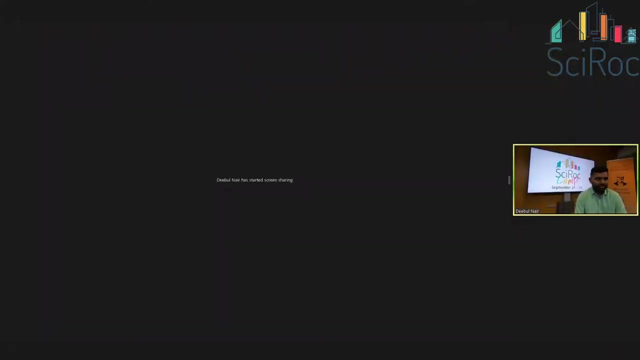 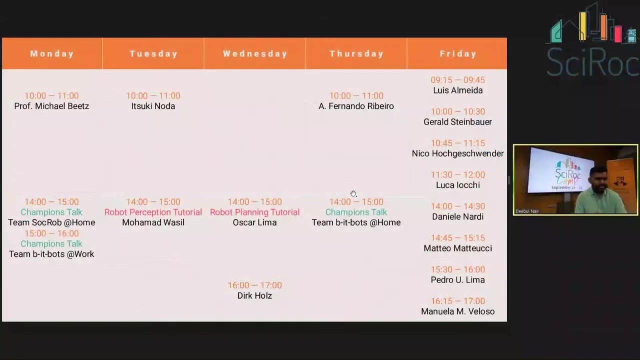 see you there. yeah, see you, ciao, ciao, bye, bye. okay, so that was uh vazil and the tutorial robot perception tutorial. so, before we leave, uh, i would like to share you what do we have for uh tomorrow, so not to forget, just a second. yes, so that's the. that's what, how it looks for the week. so we are right here today. 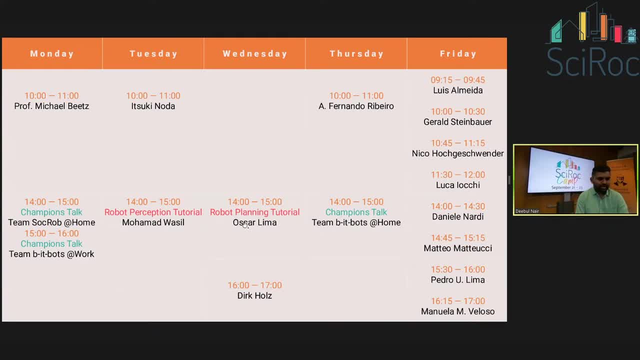 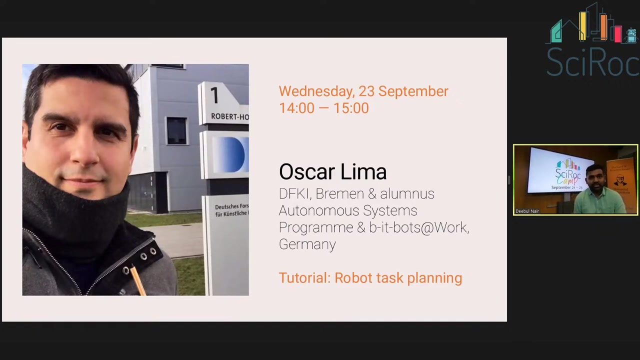 on tuesday for perception tutorial and uh, the whole week we have our uh the whole week. we have the whole um, we have the jersey symposium running around and on what is there? tomorrow we will be joined by Oscar Lima and he is giving us a tutorial in robot task planning. 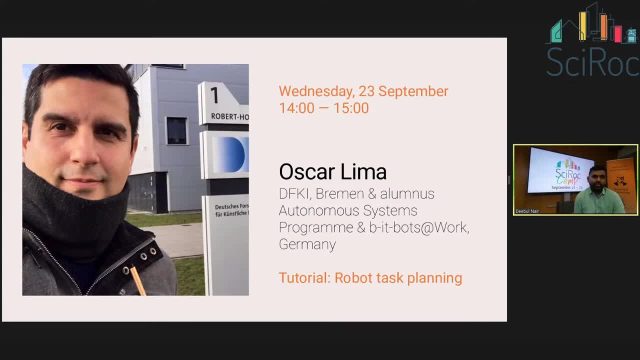 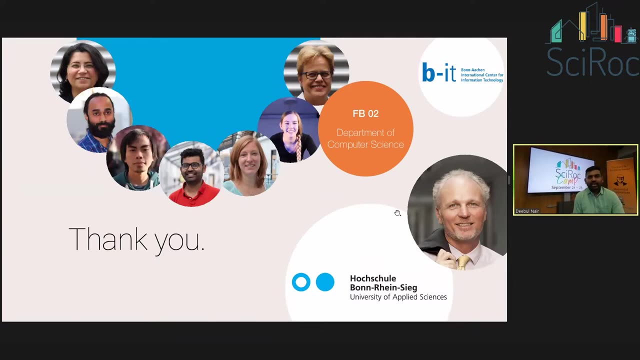 so all those questions around how does the planning in robotics work? it's a good place to start again. it's from 14 to 15, so be prepared. and finally, let me thank my team members who are helping me in there. so it's Iman Sandosh. 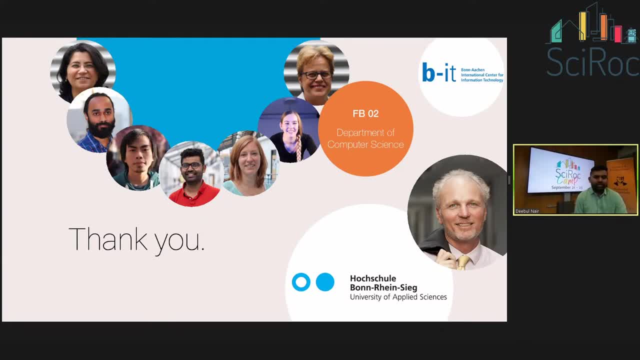 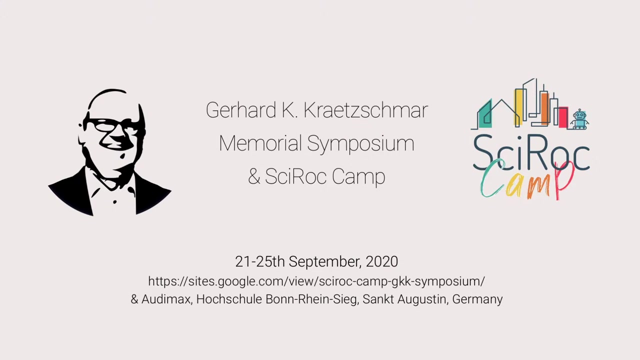 even Miriam and the whole marketing department, Kira, also our sponsors, BIT and international department here. so thank you everyone, and this is Dibu signing off. bye, bye, you. you.